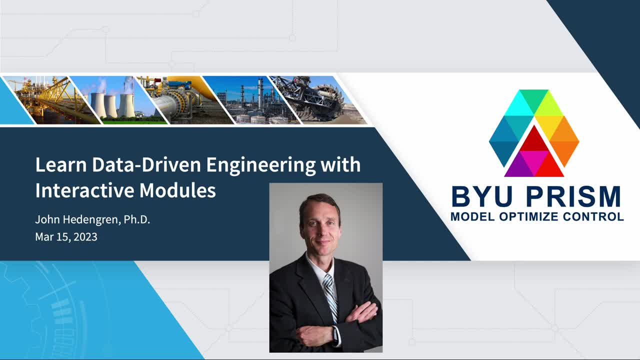 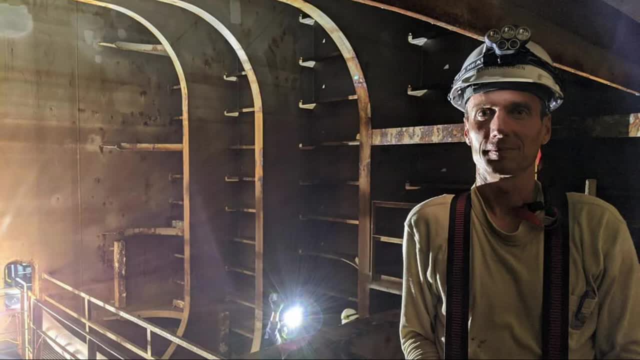 Hello, my name is John Hedengren and I'm going to give an overview of learning data-driven engineering with interactive modules. I want to start with an experience that I had a couple years ago. We went out to an offshore oil platform, Deepwater Gulf of Mexico, to install. 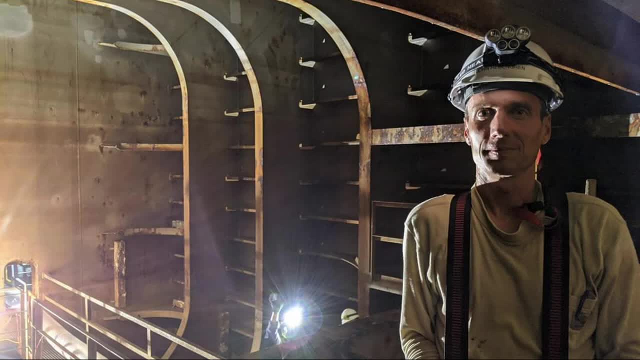 and instrument these fiber optic sensors on the web frames of this hole, of this platform, And this was about 100 feet below the sea level in these large caverns where we attempted to install these fiber optic sensors on this plate. in one of these web frames And one, 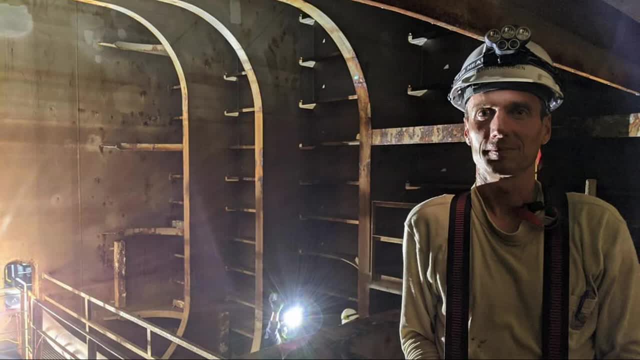 of the plans that we had was to use the data and feed it through a finite element analysis model to be able to tell the tendon tensions on the platforms. This is a very interesting technology. This is a very interesting technology. This is a tendon tension leg platform in the Gulf of Mexico. These tendons attach to the 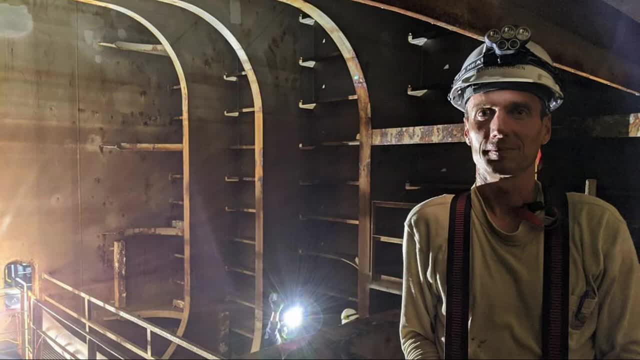 seafloor, and it's very important to be able to know the tension on these. So we used this data with this finite element analysis model, and it didn't match the load cells that were there, And so we had a decision at that point: We could abandon the project. This was kind. 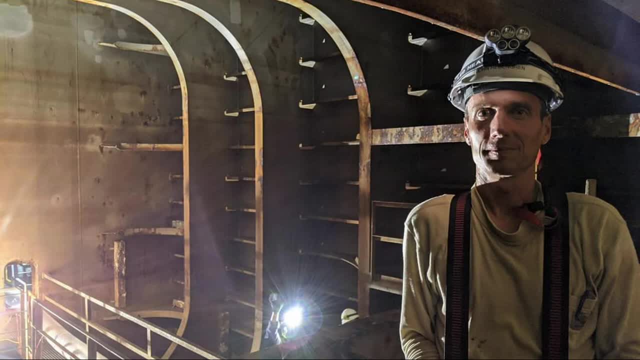 of a trial project to see if it would work or we could try some other methods. So, out of that decision, instead of using the finite element analysis, we performed a regression with the data, compared it to the load cell values and fit, and then set up the data pipelines. 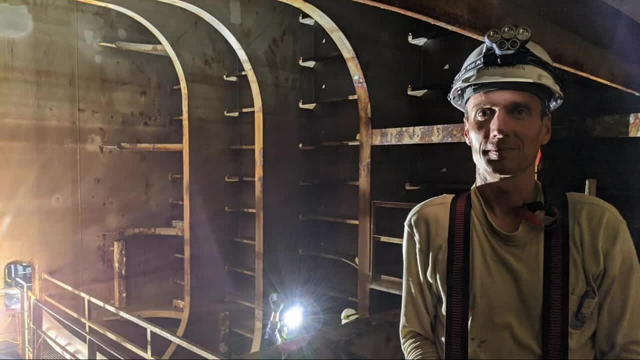 to turn that into tendon tensions and then be able to display it on an operator screen. We had to move the numbers with a SQL database and Modbus connections and all the software and systems in order to be able to take all of those raw fiber optic sensors and a fiber 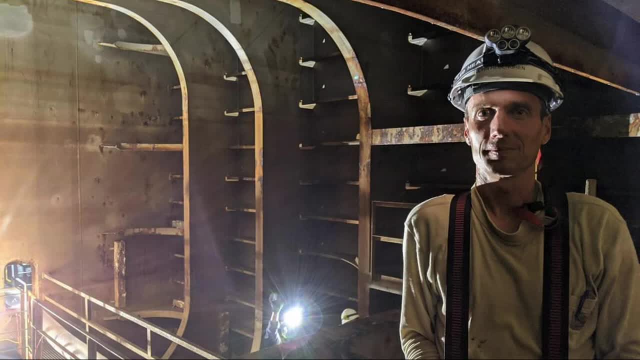 optic interrogator Running at a thousand Hertz and be able to condense that down into information that could display on an operator screen. And one of the things that we did with this is take these signals and use Python to be able to do all of the pipelines and all of the other software. 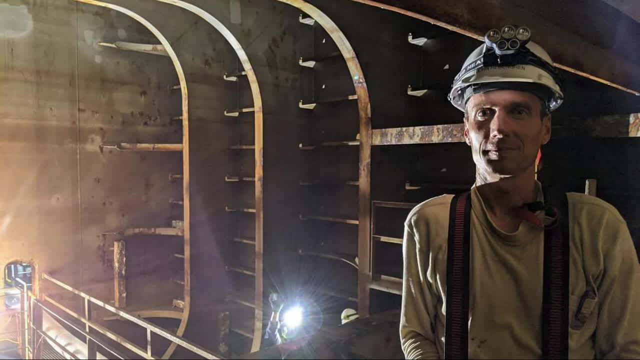 architecting. So Python was used for everything, including some of the data analysis cleansing. uh, be able to perform the regression on a regular interval, once a day, be able to re regress some of the parameters and then be able to feed those best parameters into the regression. 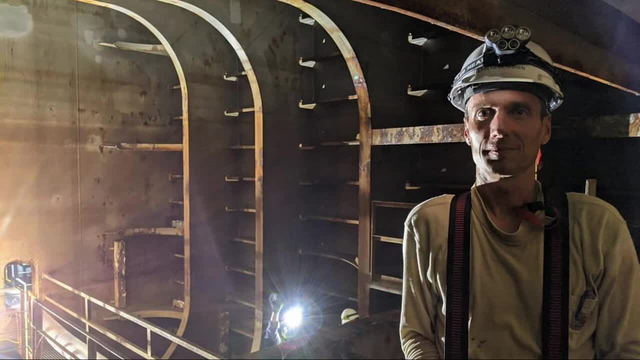 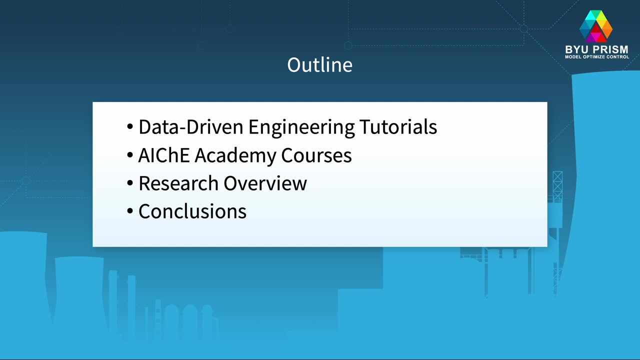 model and continuously give a prediction to the operators. So I want to give an overview of what we're going to be discussing today, And this is a lot of this is motivated by my own practical experience working in chemical plants, refineries, on offshore platforms. 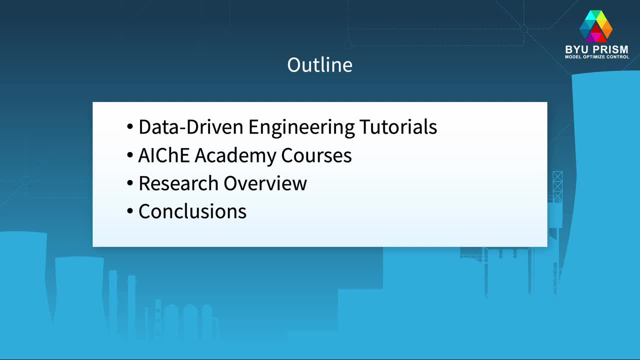 And with Other projects. I want to show you some of the data-driven engineering tutorials and also an American Institute of chemical engineers Academy courses. This is the division of AICHE, that is, is concerned with education, especially continuing education, and then give a brief. 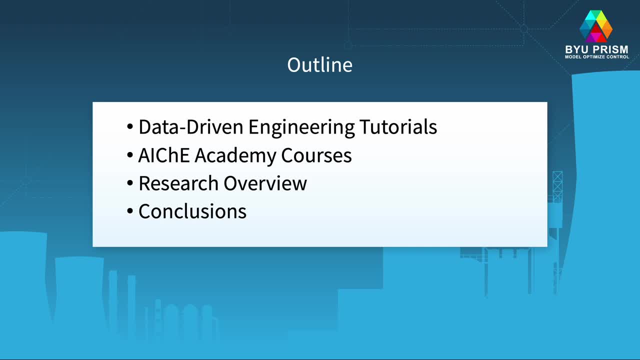 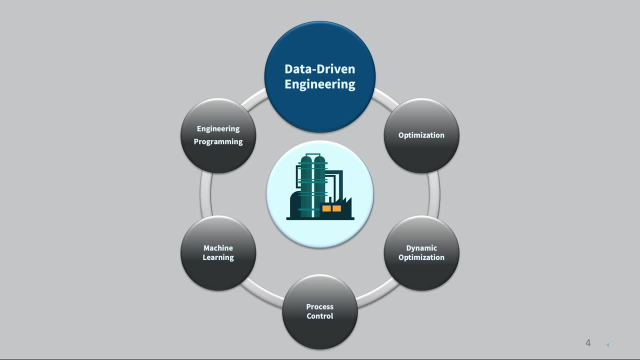 research overview of some of the other activities that I'm involved in, and then some conclusions as well. So in this one, I'm going to be focusing In particular on this data-driven engineering, and we're going to talk as well about some 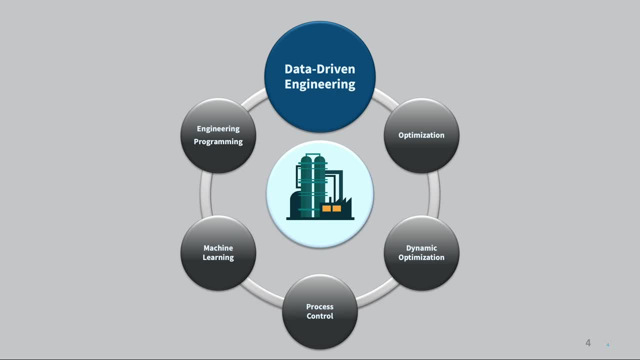 of the other courses that are there as well. There are five other courses, starting with engineering program, an introduction to programming in MATLAB or Python, also with Excel to be able to help somebody who has almost zero experience with programming, And then also the process control course. 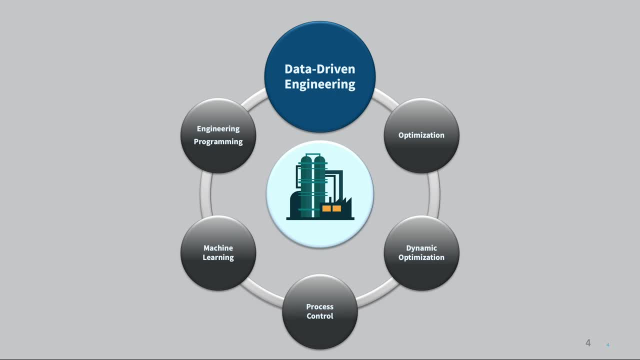 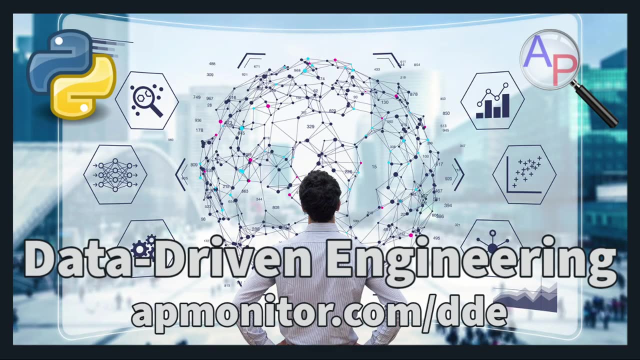 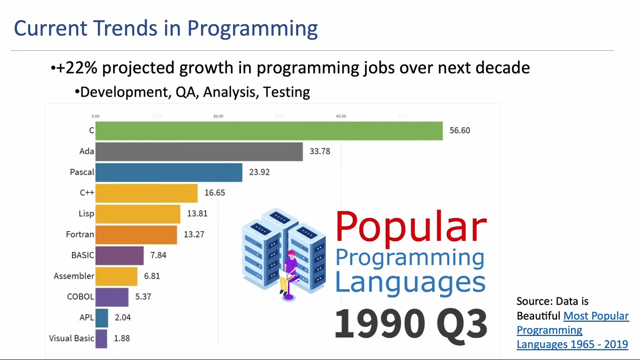 So one I'd recommend next, or optimization, And then machine learning and dynamic optimization. So this new course is apmonitorcom, slash DDE for data-driven engineering, And I'll give an overview of some of the modules that are there, And we'll also spend a little bit of time to explore a couple of those modules together. 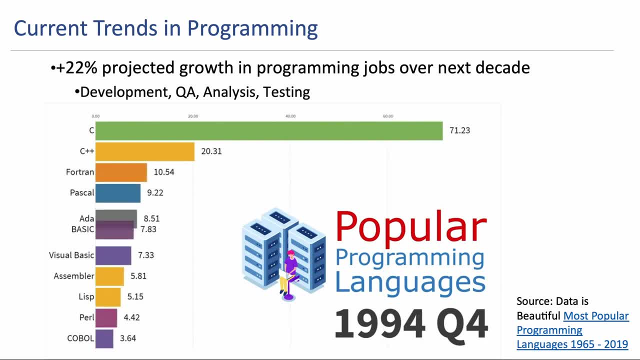 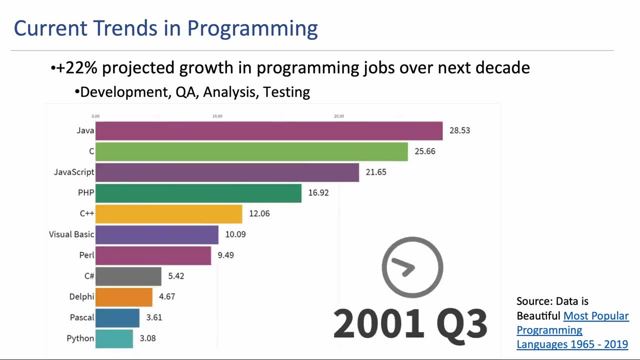 So let's just talk about some of the current trends in programming. there's projected to be a 22% increase in programming, So we can start talking about some of the most popular programming languages over the next decade, And here you can see a graphic that shows some of the most popular programming languages. 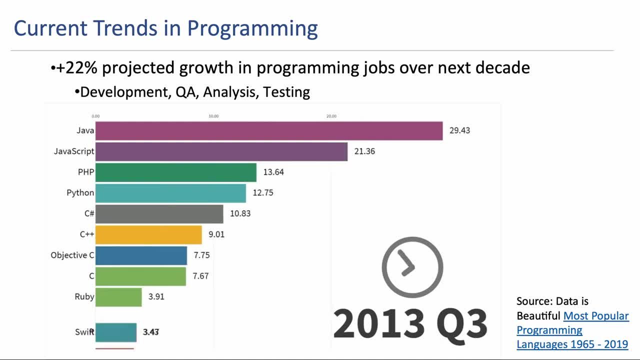 over time. Now the thing to take away from this is that the popularity of different programming languages changes. There might be a better programming language that receives more developer mind share, Also certain industries like web programming or web development. Now the interesting thing is that Python has emerged on top here, and that's also a scientific programming language. 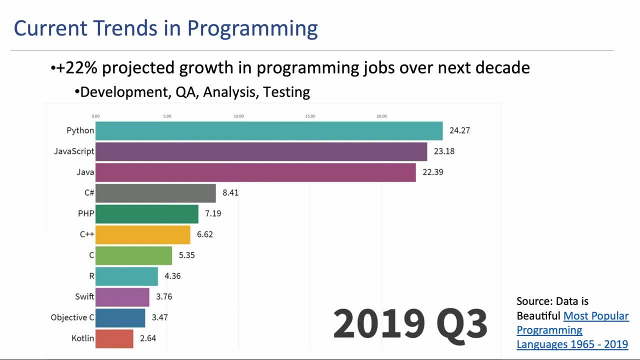 So the focus of this course and these courses is going to be really tailored toward engineers who want to be able to do engineering analysis, design, optimization, And fortunately this Python ecosystem has evolved that includes so many other things, even beyond just the engineering design and analysis. 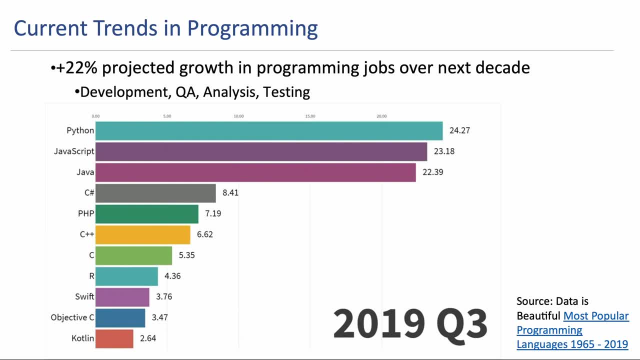 So it's like a Swiss army knife of programming languages that can even interact with others and be able to form them like a glue that holds everything together. That's part of the reason why I was able to do that substantial project with Python, because it's full-featured and helps with the data pipelining and other aspects, modbus connection and so on. 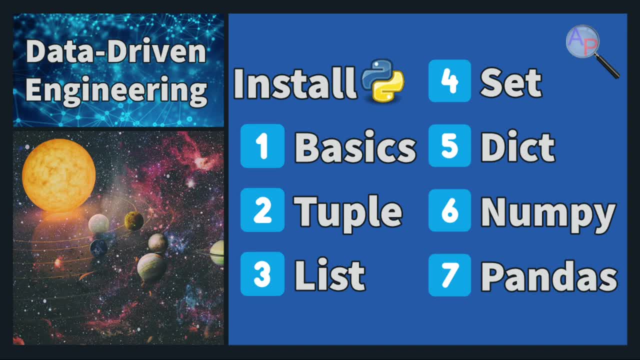 Okay, so let's just start with some of the basics. For those that are just beginning with Python, I'd recommend these seven modules: First, how to install Python. That's a critical step and some people end there. They can't get past the how to install Python phase. 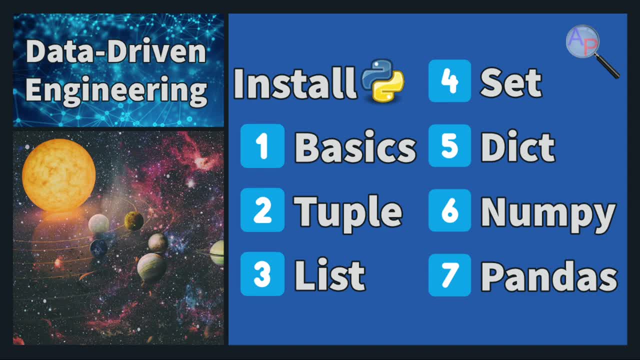 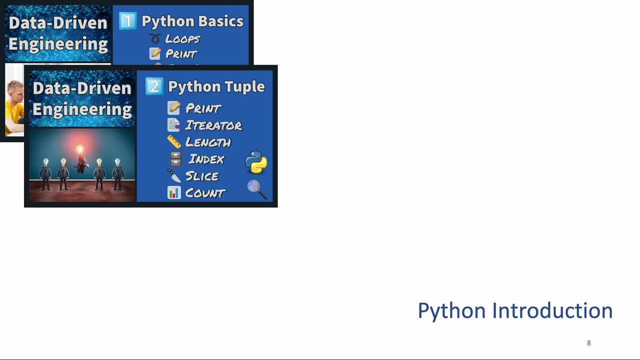 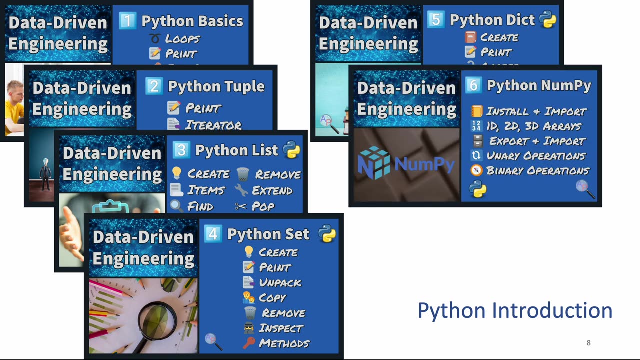 Next just basics, tuples, lists, sets, dictionaries, numpy and pandas, And for each of these there's a 30-minute to one-hour module for each of them. So Python basics, Python tuples, lists, sets, Dictionaries, numpy and then pandas. 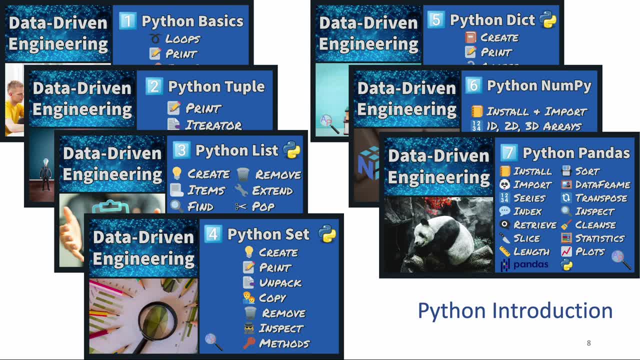 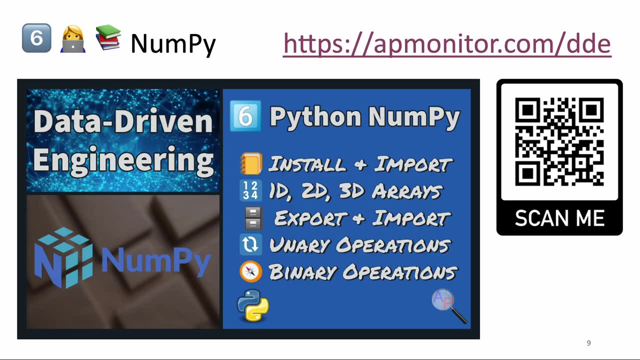 We're focusing just on a subset of Python, because Python is quite a large, has many packages and other features that are important, but we really want to focus on the things that are going to be important for engineers. So this is the Python introduction. 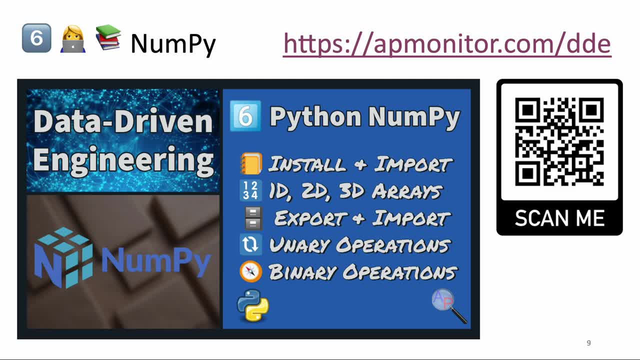 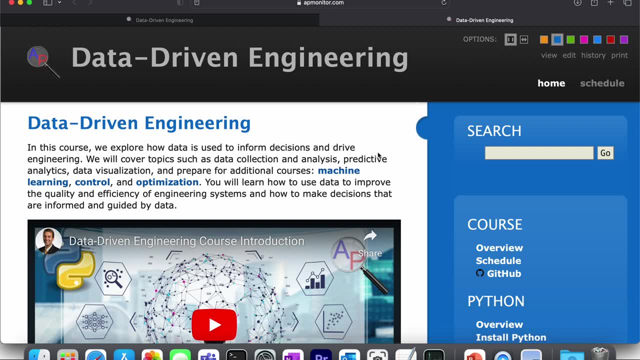 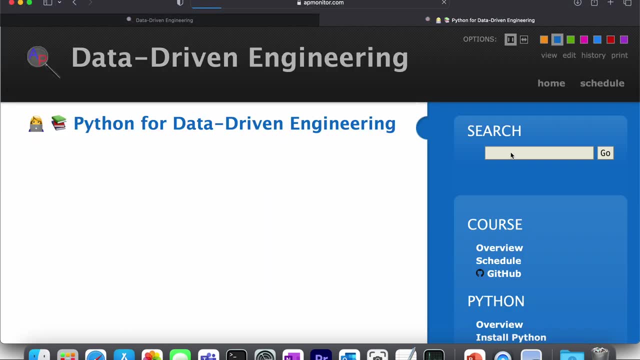 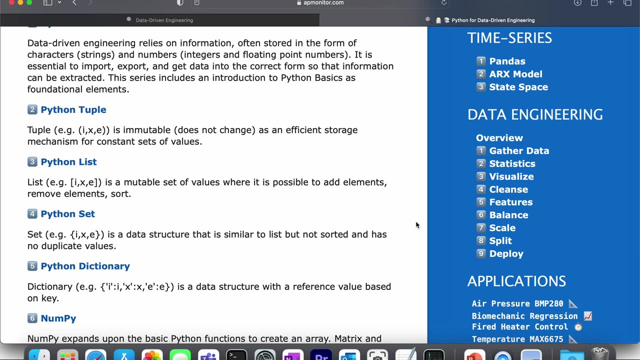 Let's just focus on one in particular. So I'm going to visit the course website. So this is the data-driven engineering course website And if I scroll down a little bit, you'll see this Python overview, And here it gives just an introduction about why Python and some of the modules that we're going to be going through. 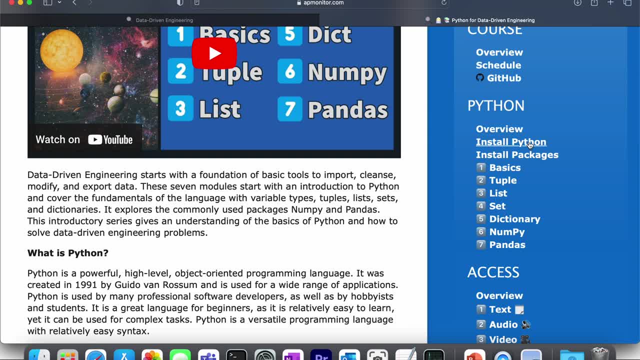 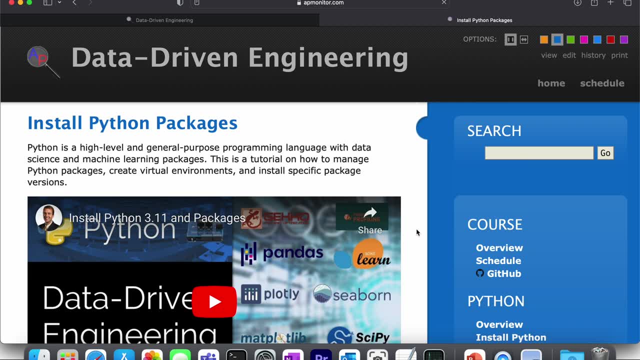 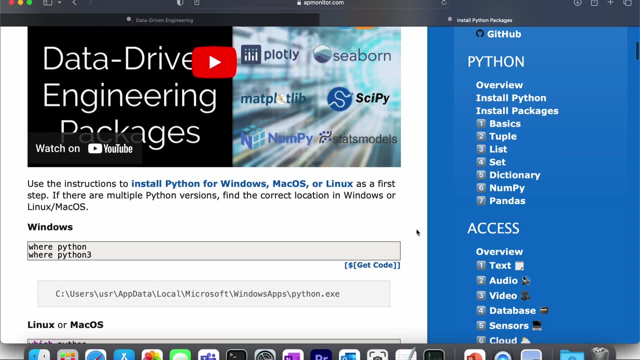 Also, I'd recommend this very first one on how to install Python, and then also how to install packages as well and be able to manage packages, virtual environments And other things that are really important with dealing with Python development. So then we go to Python basics. 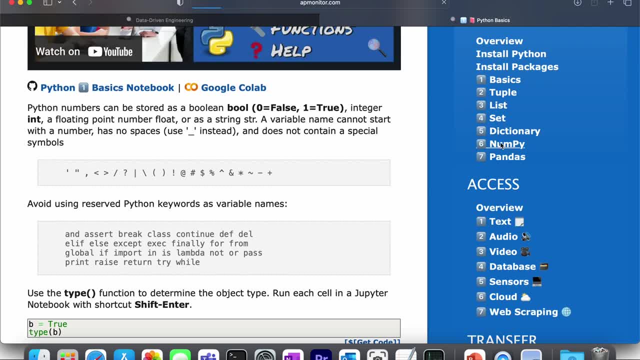 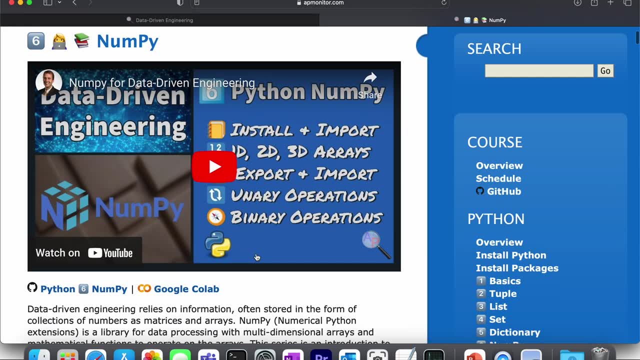 Okay, And as we go down, I'm going to go down to numpy, Just focus on that one. This is numerical Python And, as you can see, there's a video associated with each of these, And then, right underneath it, there is the GitHub link if you want the Jupyter Notebook to run through this. 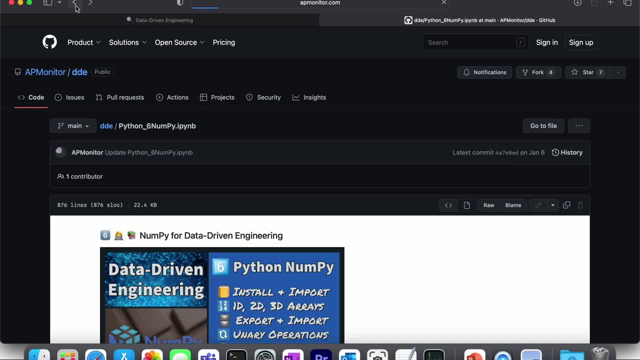 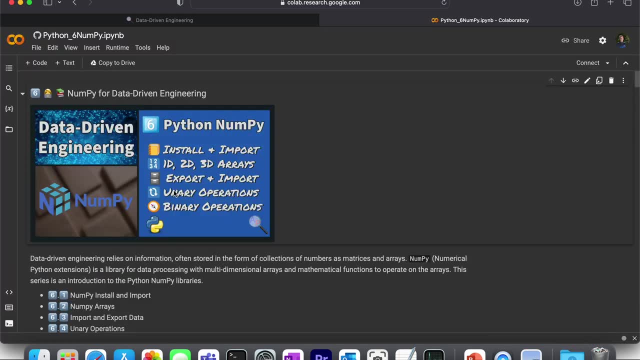 And you can download this directly And run it locally, or there's also a Google Colab link, So Google Colab lets you run it directly from a web browser or your cell phone or some other environment where you don't have necessarily have to have Python installed. 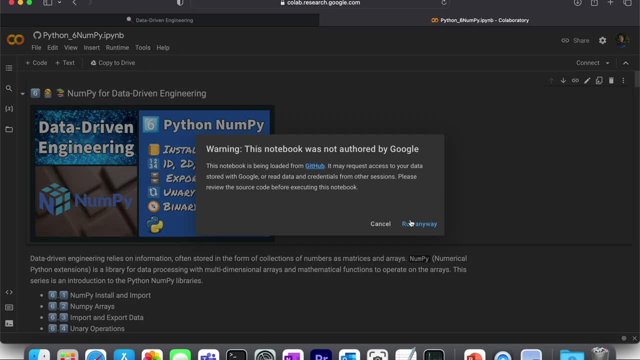 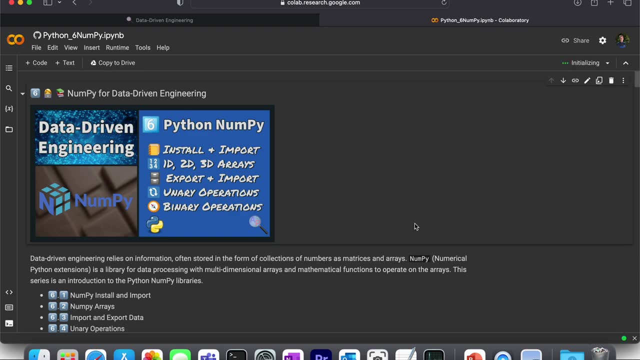 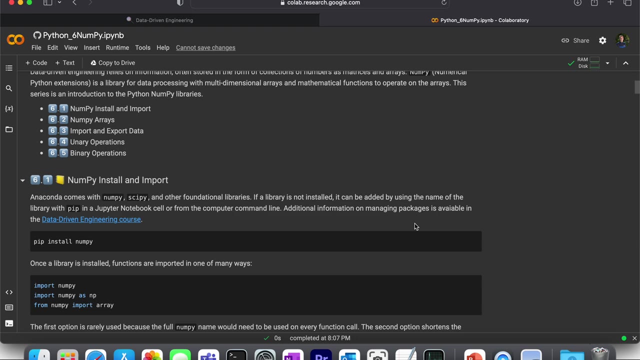 And then when you run it, I'll just go run, anyway It's not authored by Google- And then you can run through these exercises. Okay, So each one has these submodules on it On how to install and import numpy or other packages, for example. 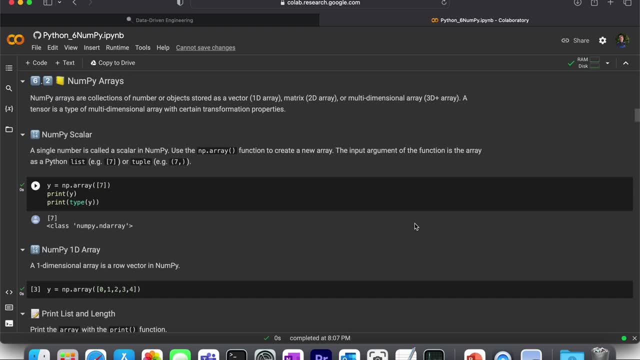 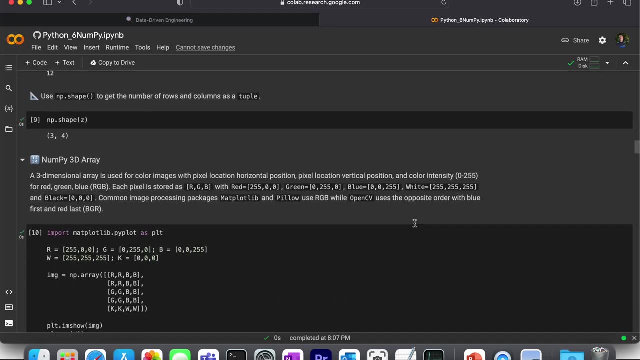 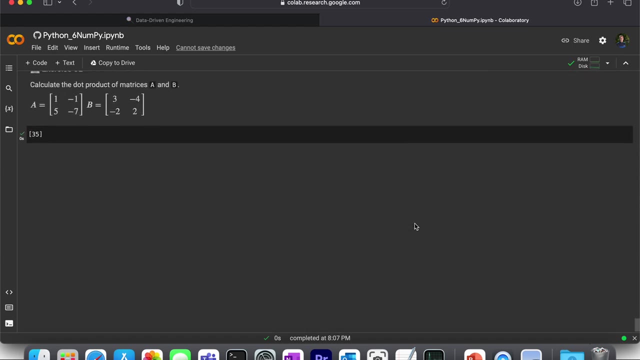 And that takes you through some of the basics on working with numpy arrays, with a description of each of those, And then at the very bottom it's going to have some activities or exercises. I'll scroll down to the very bottom here, Okay. 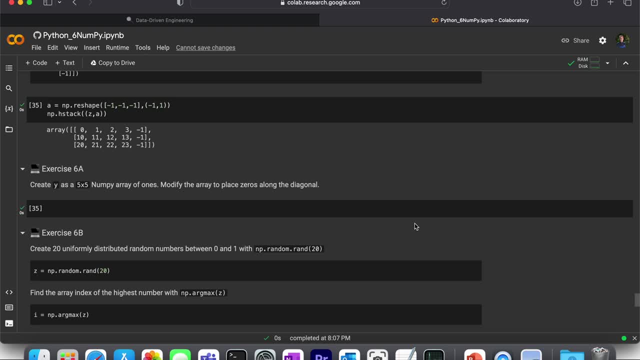 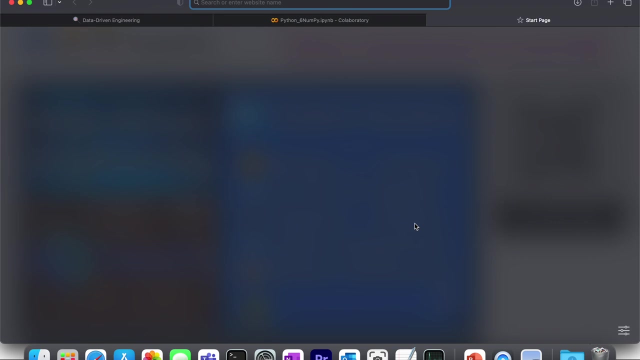 With you know exercise. it says 6a, 6b, And one of the things I'm going to show you is: if you get stuck, there's different ways to find help. A very good way to do this is stack overflow. 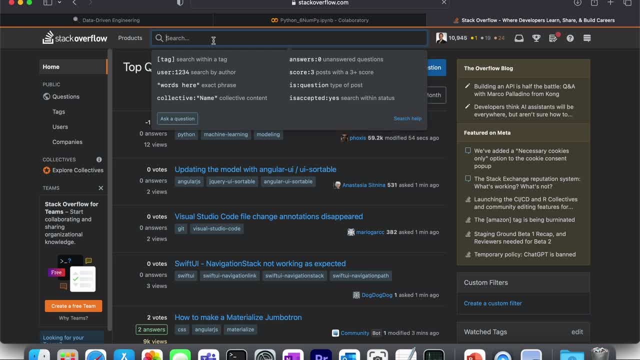 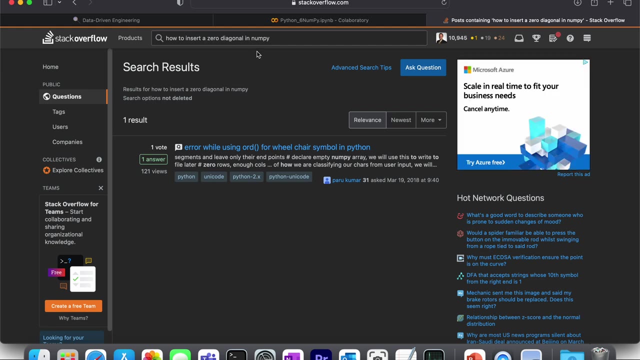 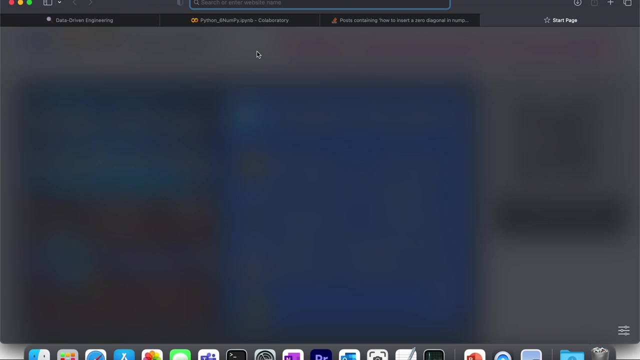 So, if you go to stack overflow and search for how to insert a zero diagonal in numpy, Okay, You might find something helpful. You can also go to the documentation As well. another way to do this is, uh, through the large language models, and these are evolving very rapidly right now, but they're also very useful. 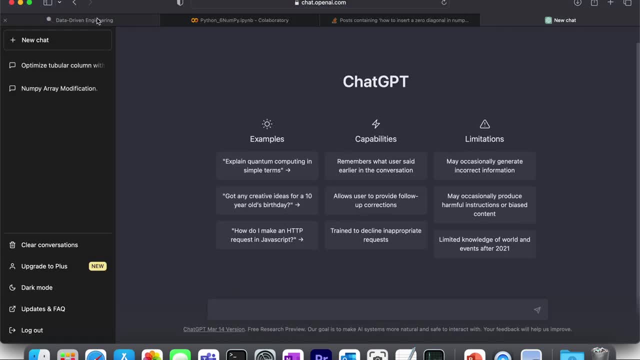 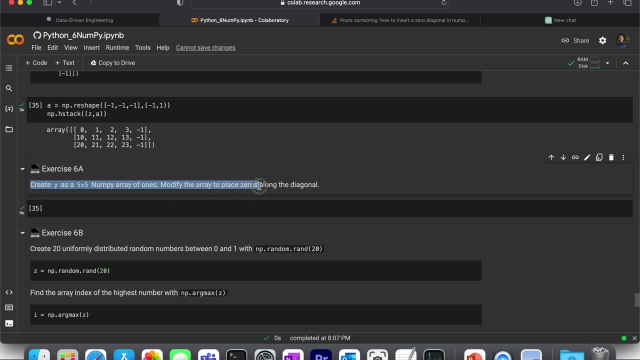 So I'm going to go to aicom and then I'm just going to type in this prompt: create Y as a five by five numpy array of ones. modify the array to place zeros along the diagonal. So I'll go ahead and copy that prompt. 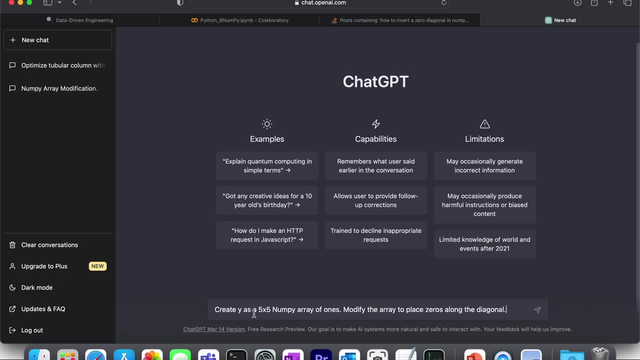 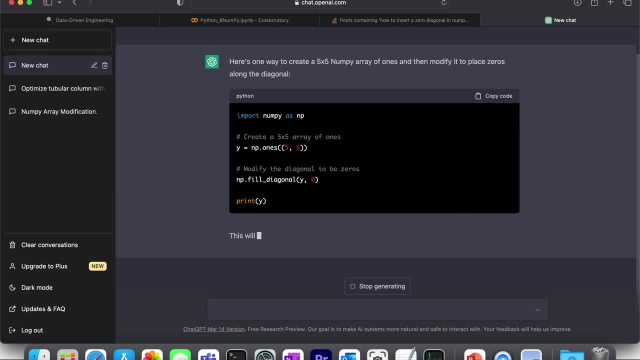 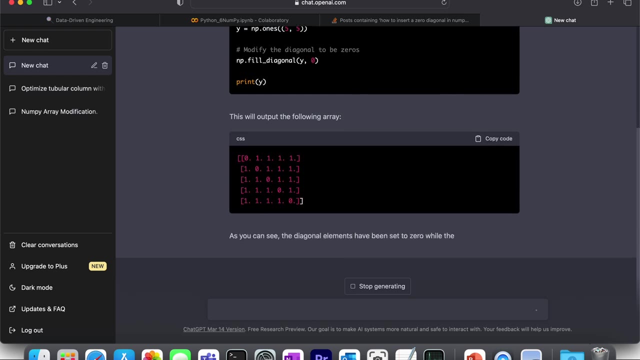 And then paste it in here and see if it can give me some help on this problem. Okay, So there are many ways to do this, and here is one way: you create an array of five by five ones, and then use the NP dot field diagonal with zeros, and it's going to output that following array: 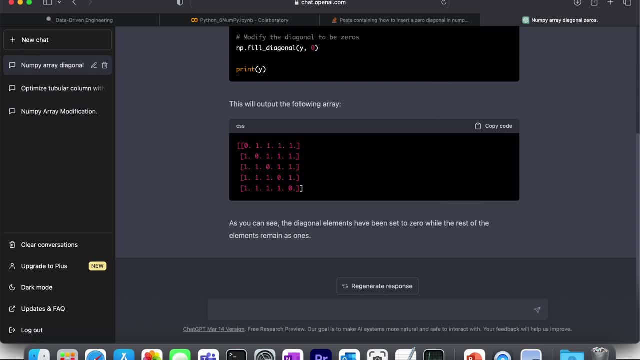 So this is one correct way to do that. The other thing is, if you have a bug in your code, Okay. So what is the error? This Python code: All right, And I'll go ahead and put in some Python, Oops. 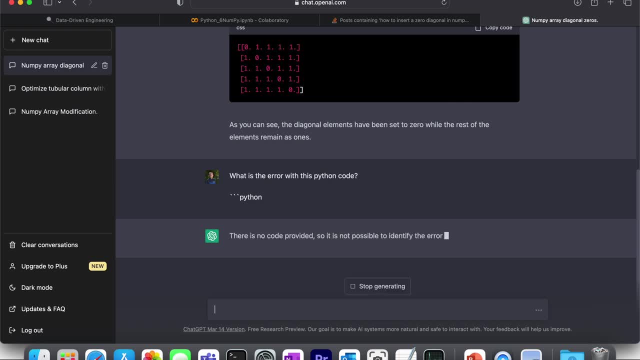 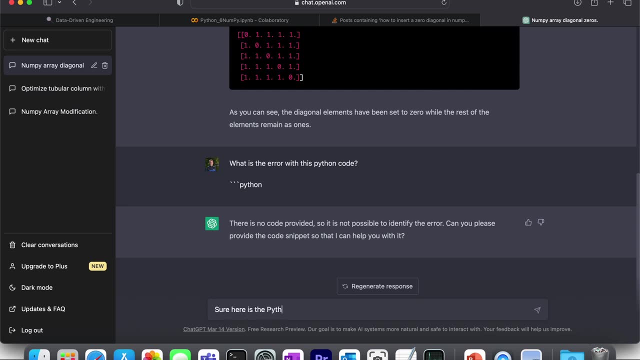 I made a mistake on that. I did it too fast, Okay, So go ahead. and uh sure, Here is the Python code. I need to hit shift, enter. Okay, And then let me go ahead and put an air in here. 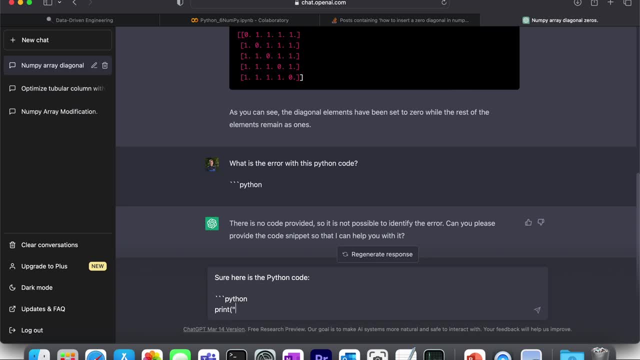 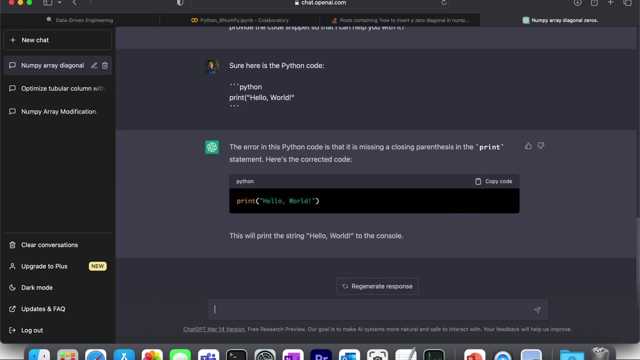 Okay, I'll leave out the closing parenthesis. all right, the air in the code is is missing a closing parenthesis in the print statement. Here's the corrected code. So in learning Python, this is going to be another tool. If you can use it effectively, it can give you immediate feedback as you paste in code. 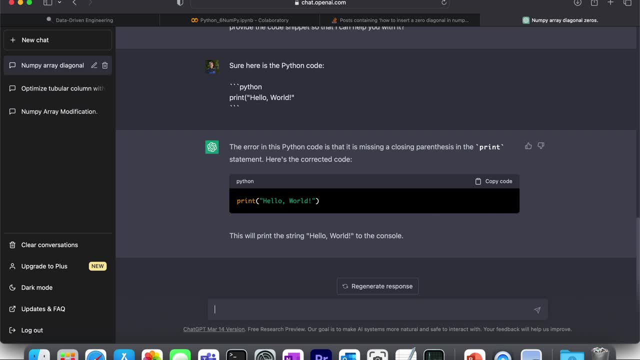 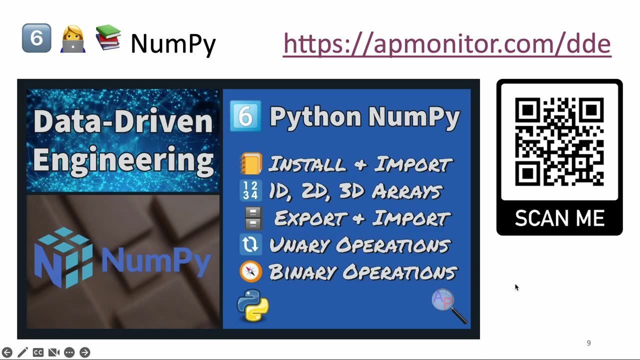 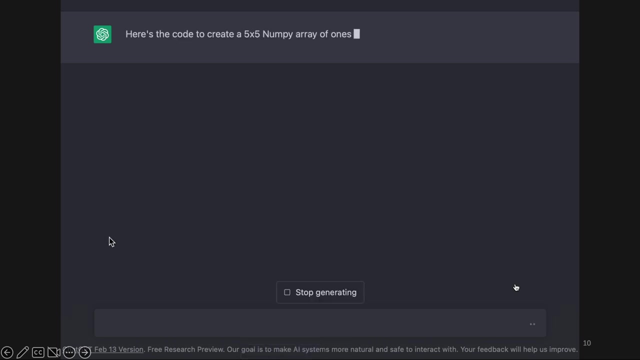 Or ask it for a little bit of help on some of these modules. I recommend that as well. Okay, So let's come back here to uh this. this is the module. This just shows the same thing with this: uh, five by five NumPy array of ones. 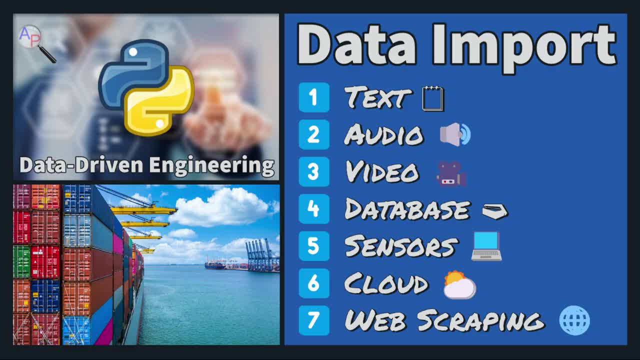 Okay, And I recorded that one before, but it's the same thing. Let's go on to data importing. Okay, Text, audio video, database sensors, cloud And web scraping. So, after we have some of the basics of Python, one of the things that's very important is: how do you retrieve data into the Python environment, be able to work with it and then potentially export it as well? 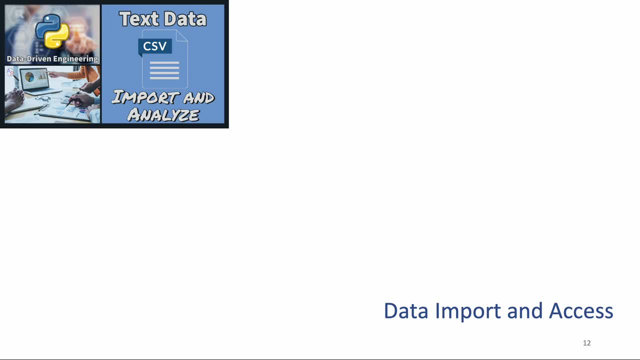 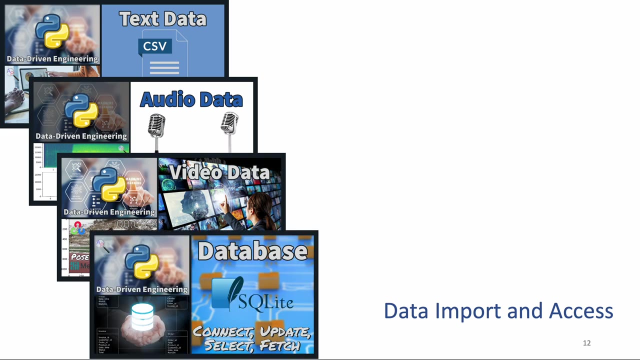 So first thing that we want to do is text data. It's very common comma separated value files, ASCII text text document somewhere that we want to be able to import into Python. Then we'll talk about audio data as well: Video data databases, how to interact with them, primarily through SQL light. 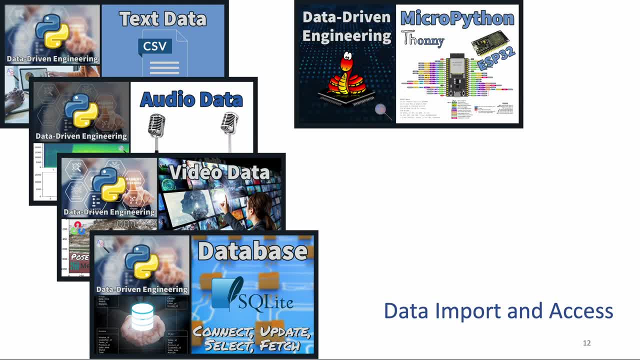 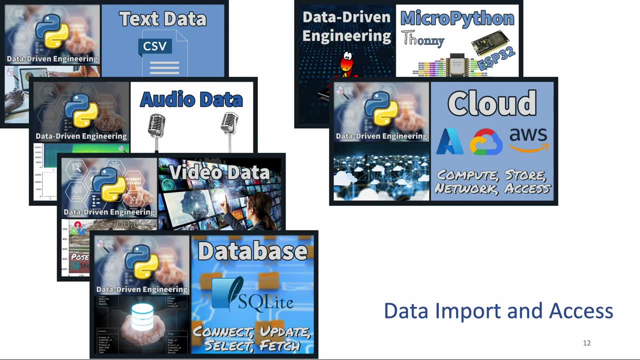 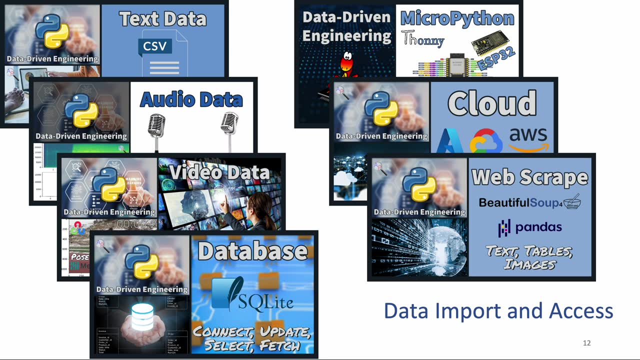 Okay, SQL light, And then we also have micro Python to be able to run on embedded devices, cloud processing with Azure, Google cloud or AWS, and then also web scraping as well, So a range of ways to be able to interact with data, both in the cloud locally on it. 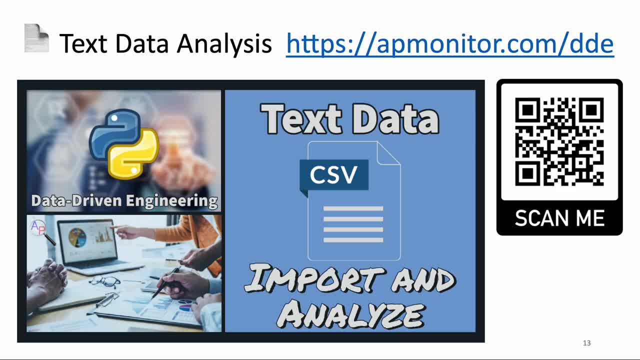 We can do that by using embedded devices and with a variety of file formats. So let's just take a look at our text data analysis. So I'm going to go back to the course where you can scan that as well for the link. Okay, 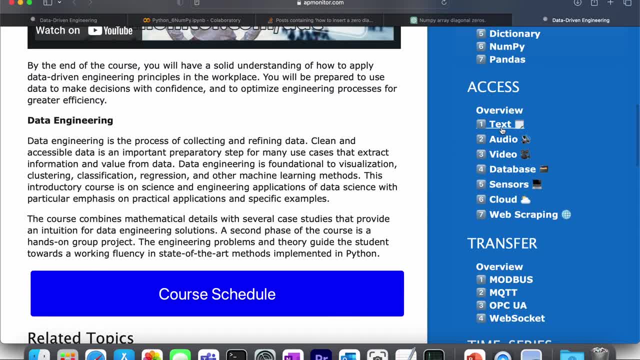 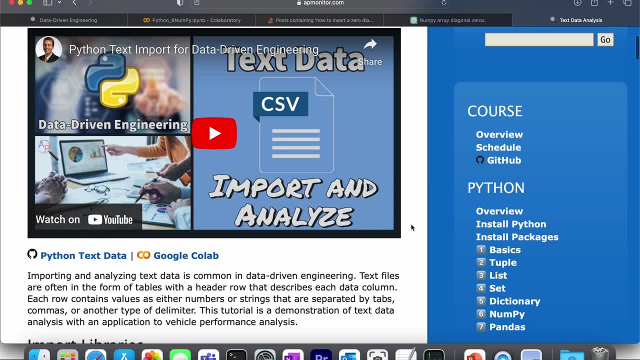 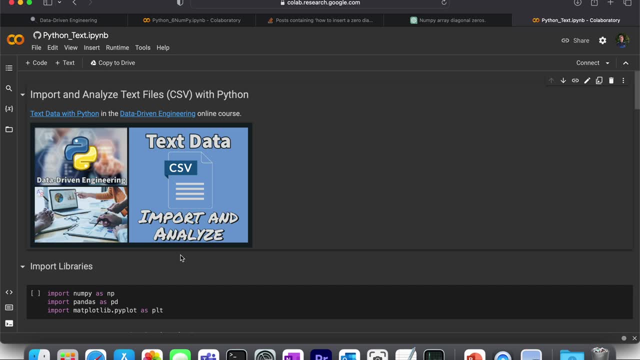 And I'm going to come here to the text analysis. Just give you an idea about what we're doing with this module, And as I scroll down I'll see this Google collab link again. I'll go ahead and select it Now. in this module, we are actually collecting data from vehicles and then analyzing it, and it gives some instructions. 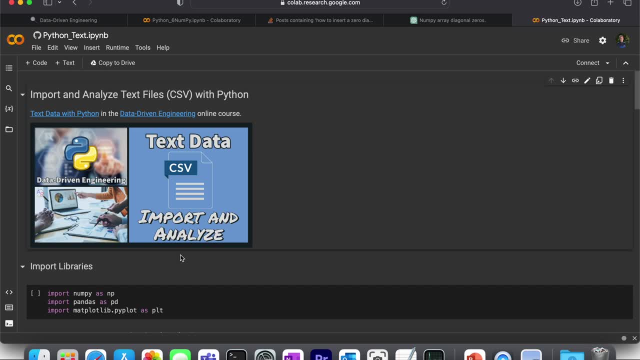 If you want to be able to collect your own data from your own vehicle through an OBD two connection in your car, there's a little $7 module that you can buy that will be able to connect to your vehicle and you can collect your own vehicles data or you can use the ones that are here as well. 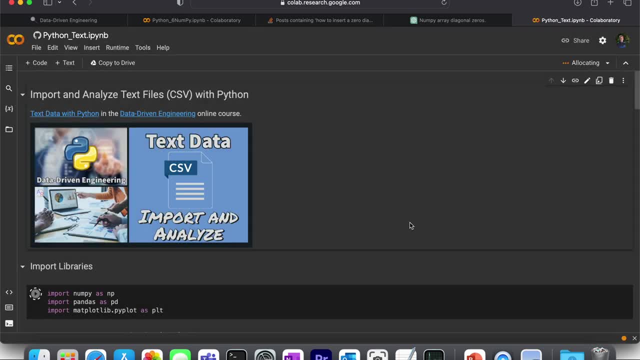 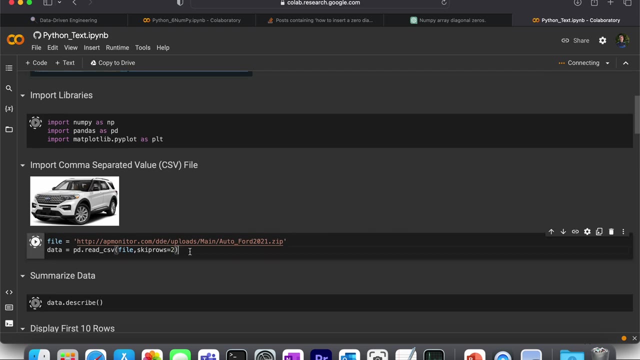 Okay, I'll just go ahead and run all So it shows what we can do with importing text data and analyzing it, And the most important part here is going to be just reading this data file. Okay, And I'm going to do that with a pandas: read CSV and I'm going to read it from a zip file. 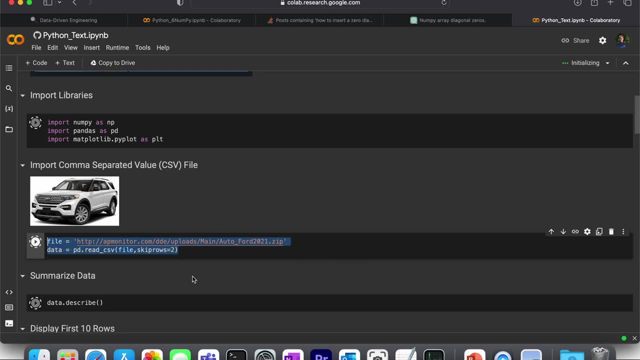 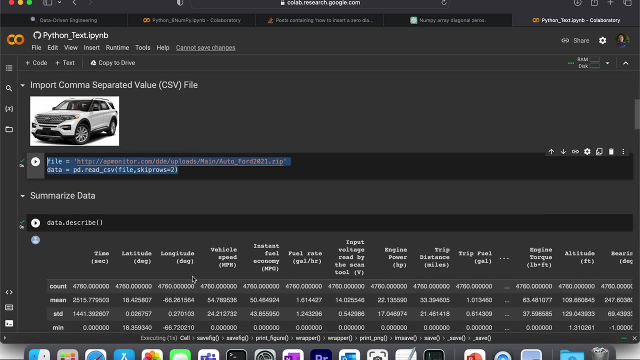 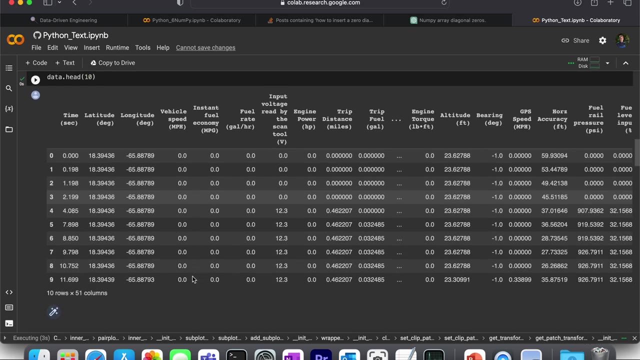 In this case I'll skip a couple of rows and then I'll describe the data. All right, So first of all, just importing some libraries. It described gave a summary, statistical summary, of the data, As I look at just the first rows of that. 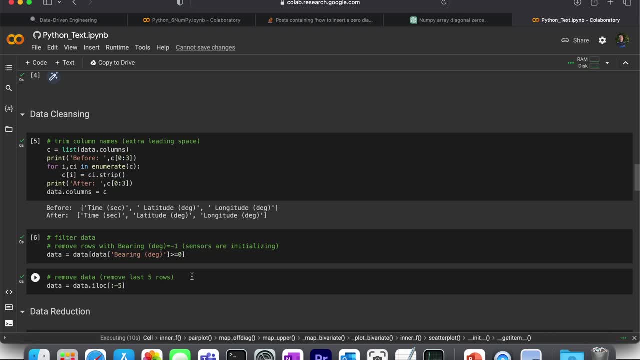 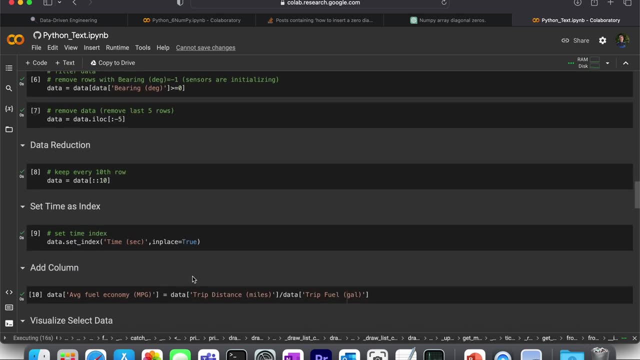 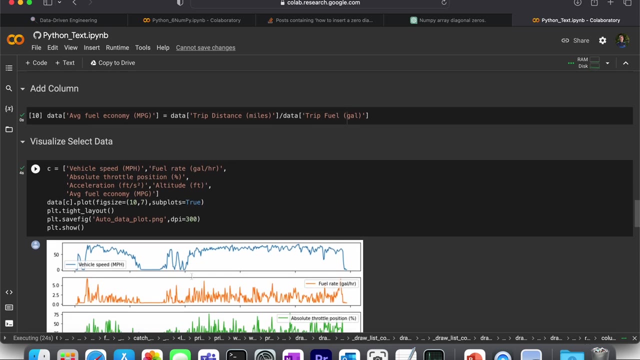 Okay, I'll do some data cleansing as well, Go through some process of removing some of the bad data, Do some data reduction like take every 10th row, set the time index And also add a column, maybe a derived calculated value. 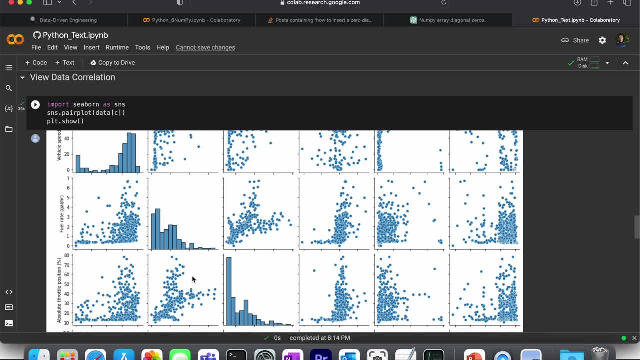 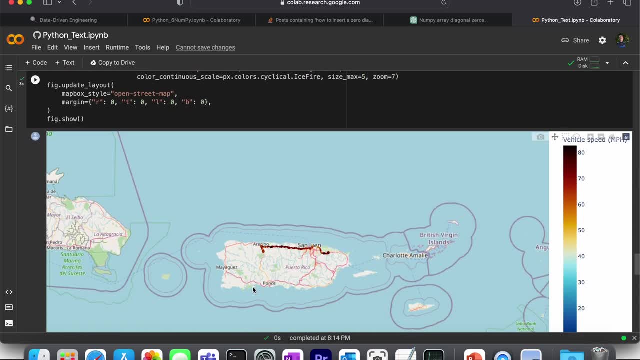 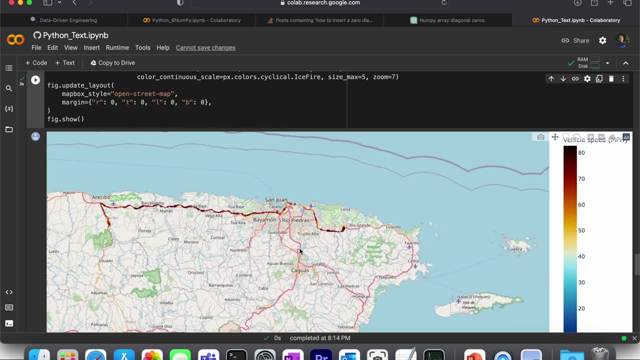 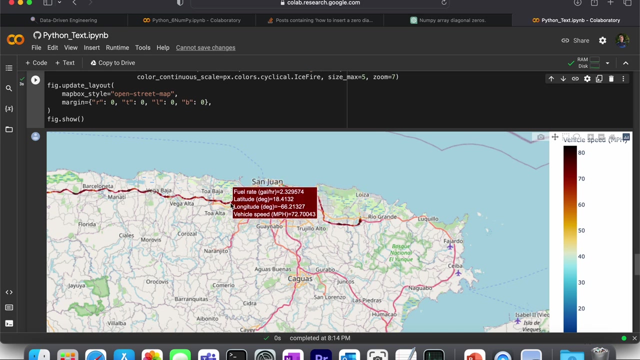 Okay, Visualize the data, View some correlations in the data And maybe there are some GPS coordinates in the data as well. So here's an example of how to create an interactive plot from that data as well. So you can see a vehicle trip here that was recorded and you can see the speed, the fuel rate, the latitude, longitude as well. 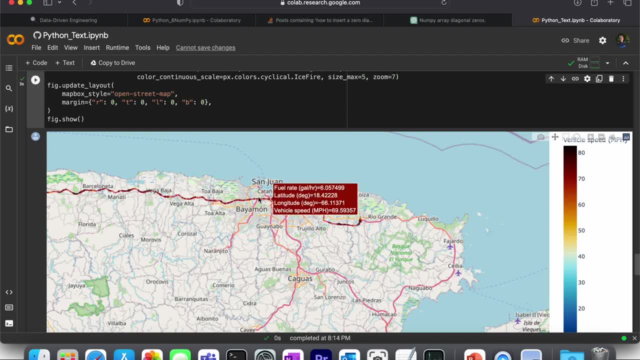 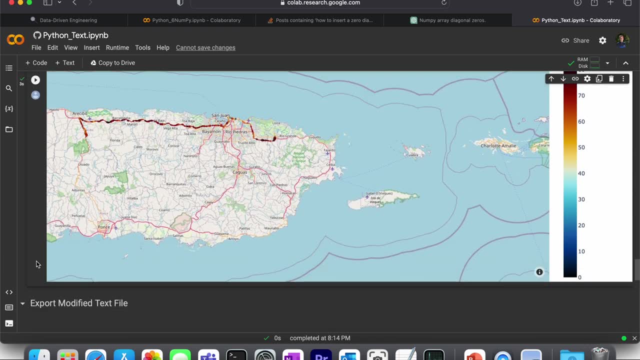 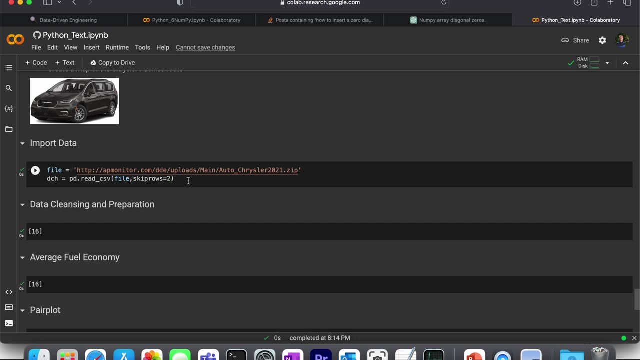 Okay, And this, And you can see the trip. So you can do this for your own vehicle as well and track your location, All right. And then there's an activity here. So this one, this next one, is just another data file, different vehicle, different location. 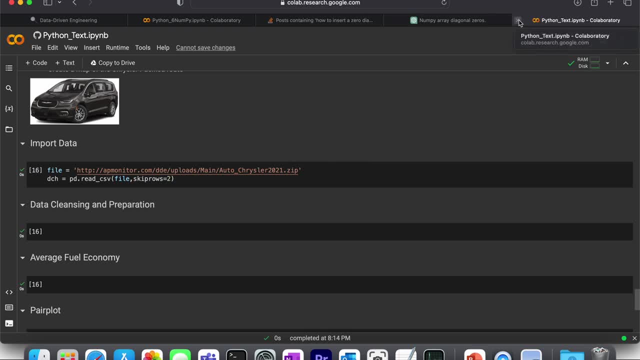 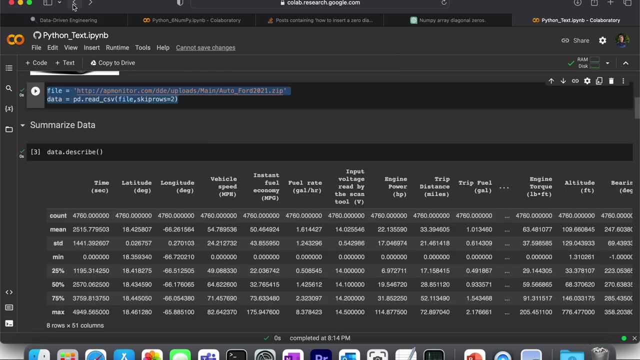 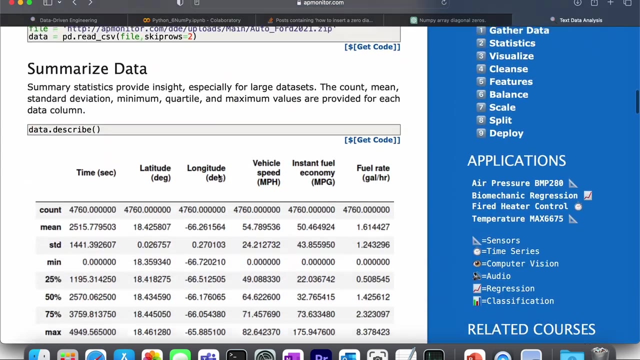 And you're asked to compare the two. Now, in this case, there's a solution video. Actually, I'll go back to that webinar Page, All right, And if you come up here to the top, there's a solution video that'll walk you through the solution. 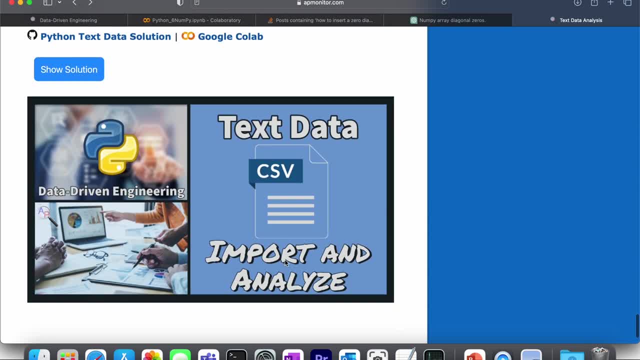 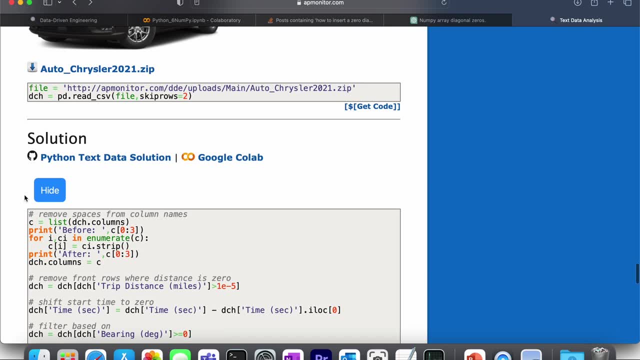 And in fact down here at the bottom there's also another video or another solution file. You can just click the show solution here, All right. So lots of solutions, lots of helps to be able to help you through that. You can also. 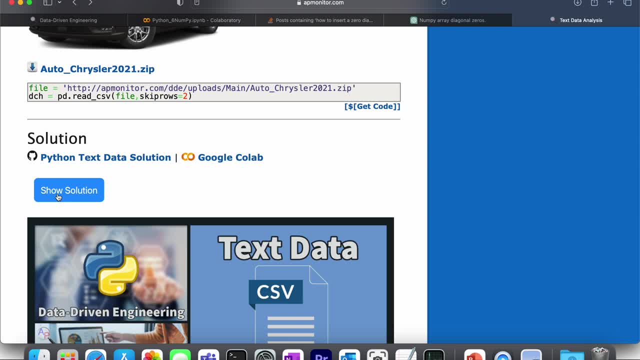 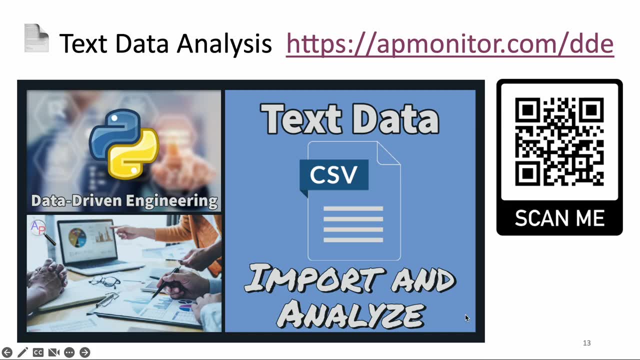 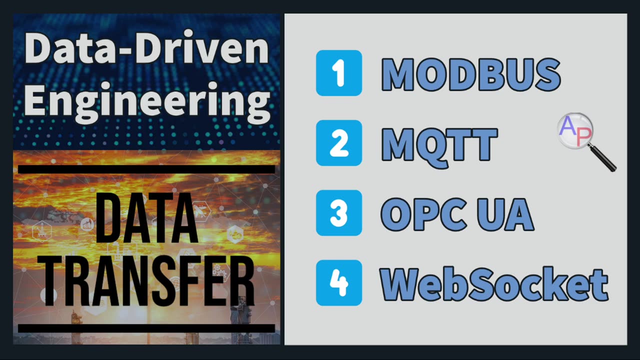 Use something like chat, GPT or stack overflow to be able to help find answers to these questions. All right, Let me come back to the presentation. All right, So after we've installed Python, know the basics of Python and also have been able to read data in. 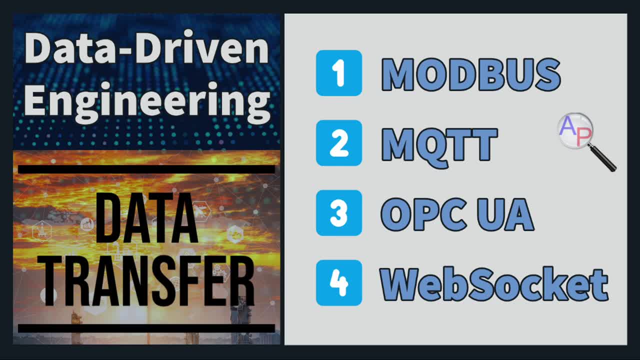 There's also an element of data engineering, about moving data from computer to computer and doing that with a variety of tools. Okay, So one of the things that we're going to talk about today is a little bit of a little bit about the, it's universal architecture, and then we also have kind of a lower level web. 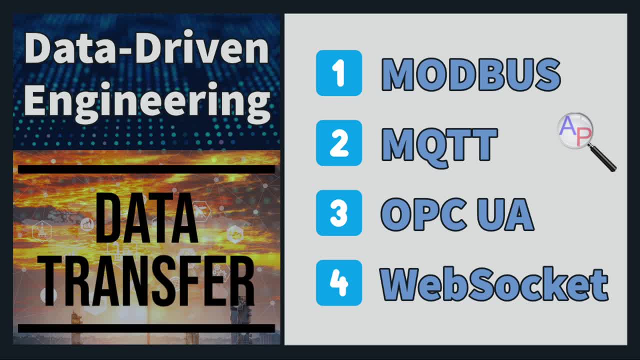 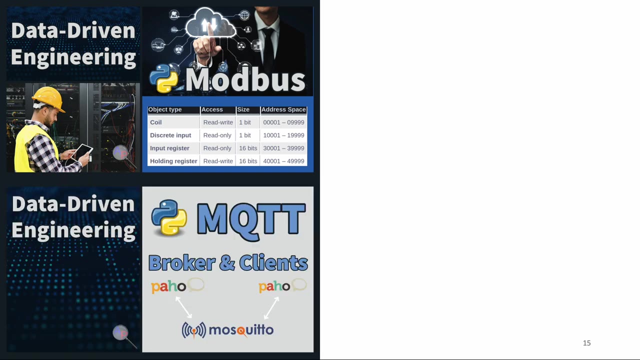 programming called web socket, but there this also introduces to some rest api's. there's some other protocols as well. they're more common with web developers and app developers and we don't cover those, but we give an overview of them just to make you aware of them. so Modbus, MVTT, sitting at the broker and 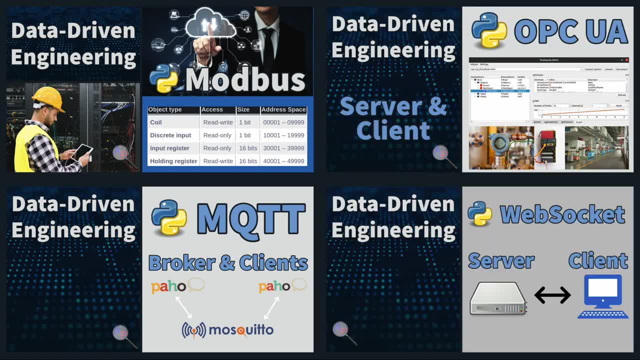 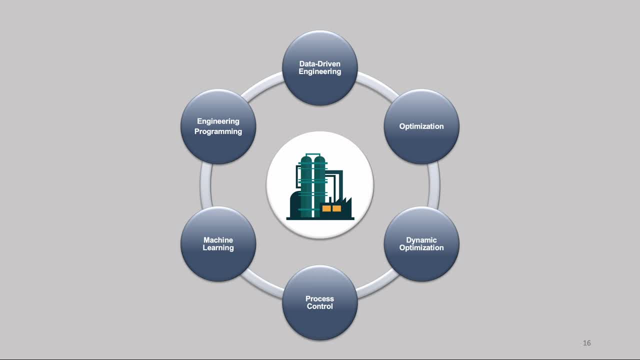 clients, opc, UA and then websockets. so let me give an overview of some other courses that are available here I'll talk about. you know, we've talked about data driven engineering, but I'd like to also introduce some of these others as well, like engineering programming, machine learning, optimization. 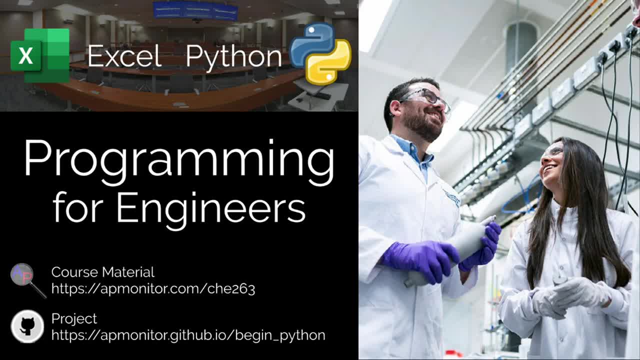 process control and dynamic optimization. so programming for engineers. again, that's a introduction to programming for somebody who's just beginning, maybe has an engineering background, that wants to be able to use tools like Excel and Python to be able to solve problems. and there's also equivalent exercises in 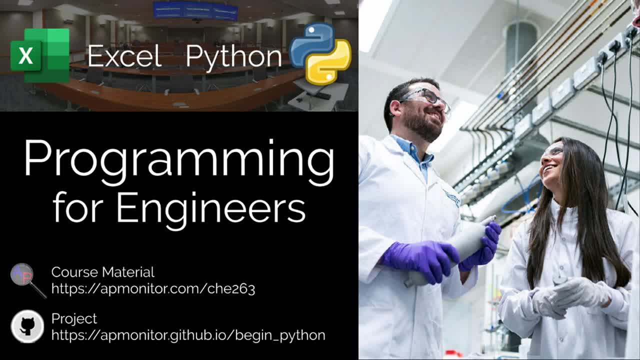 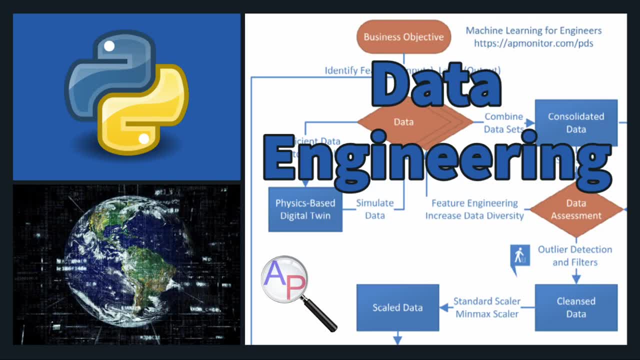 MATLAB as well. so for each exercise you have Excel, Python and MATLAB solving the same problems. next is data engineering. data engineering is really the process of taking raw data from sensors and getting it into a form that's curated so that you can do machine learning and data visualization- other activities. so 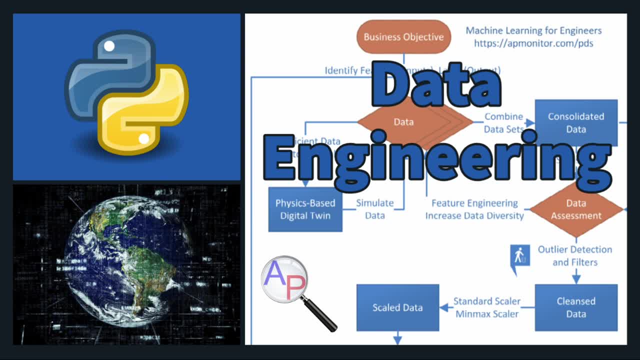 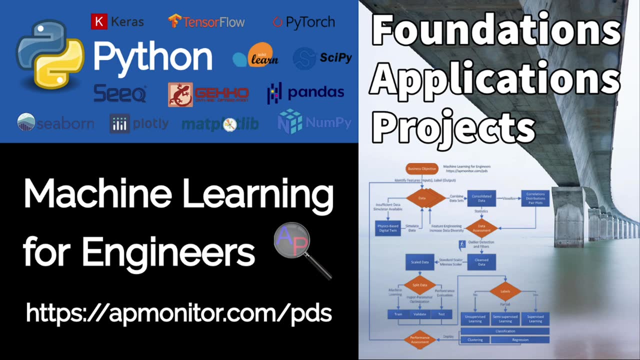 it's really this front end of the process and be able to create valuable data, and then we're going to look at the machine learning phase. so machine learning is gonna be the next one. so machine learning for engineers is really focused on case studies that are relevant to engineering. for 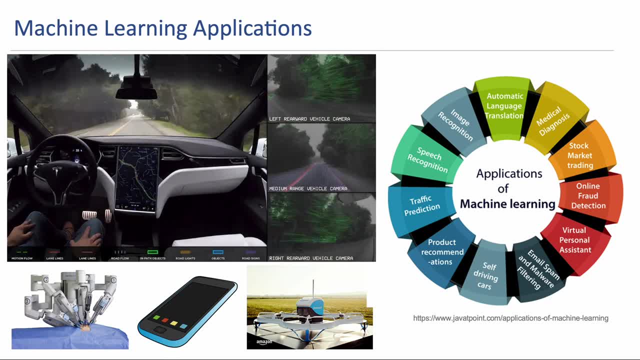 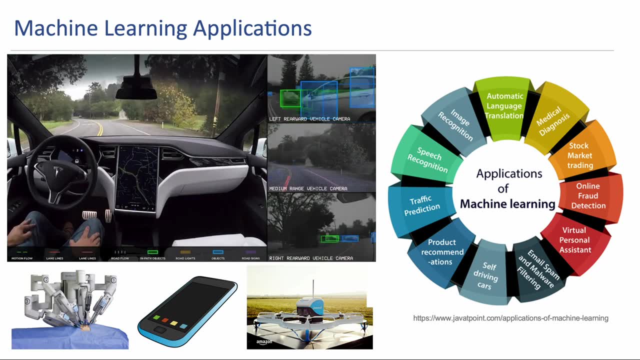 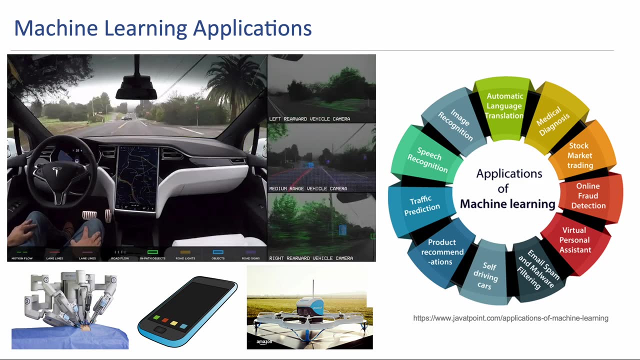 classification and regression. now, as you look at this self-driving car, you know that a lot of engineers worked on this to be able to enable this driver or this passenger, really not touching the steering wheel, to be able to arrive at a destination without guiding the car. 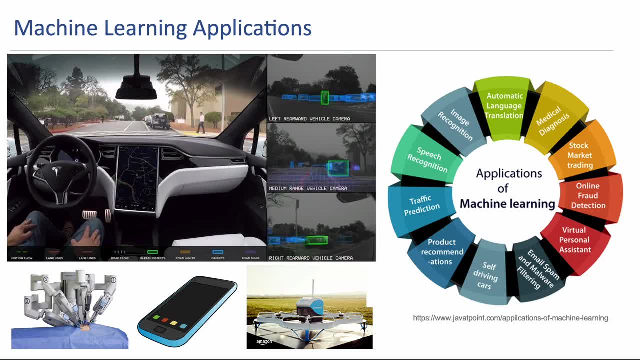 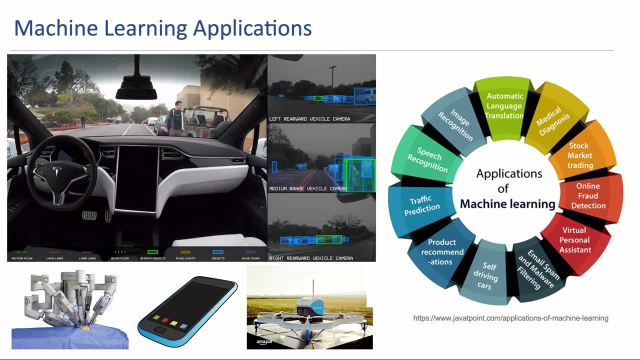 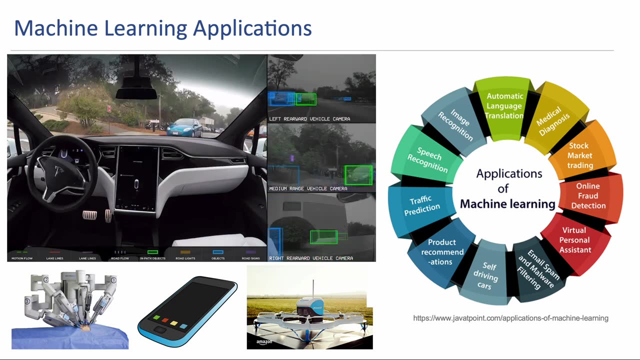 And you can see on the right some of the classification that's taking place with the computer vision from the different cameras. Then the driver leaves the vehicle and requests that the car go find a parking spot. The car is able to go into an autonomous mode, find a parking spot and be able to parallel park. 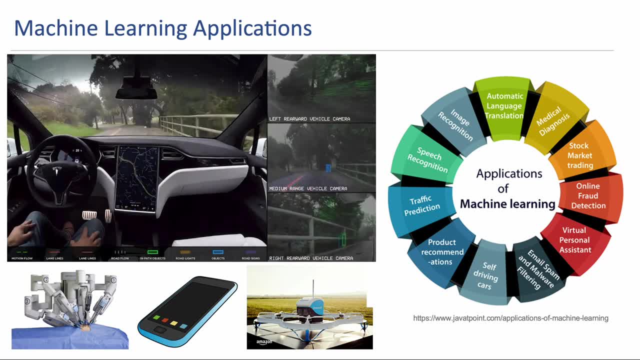 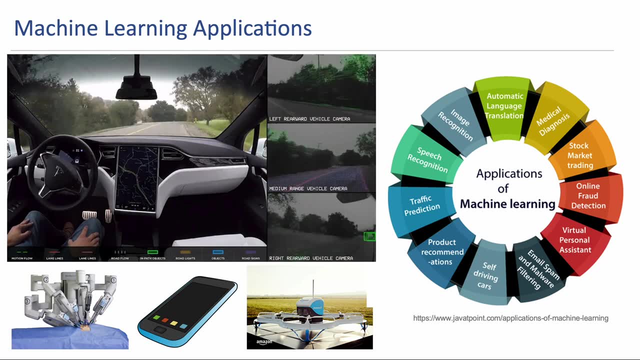 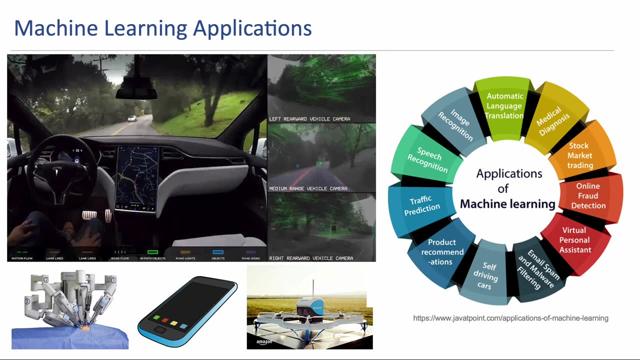 So, as you think about machine learning applications, you think about many that you interact with on a daily basis, such as email, spam and malware filtering, online fraud detection. with your credit card, You might have speech recognition that you use on your phone, image recognition and many others. 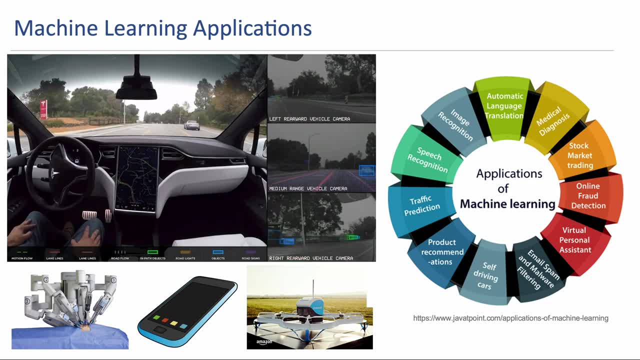 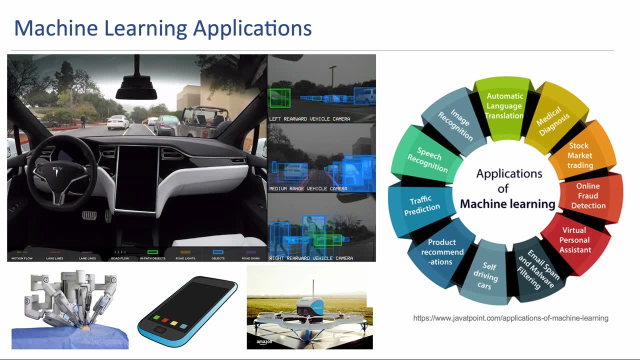 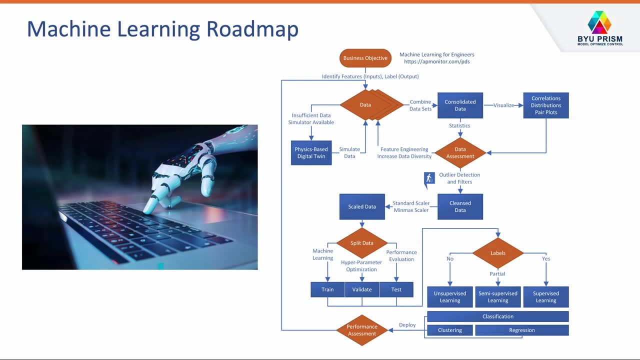 And these examples are going to be increasing as well. I mentioned some of the large language models and how those are going to start. They're appearing in some more products that we use on a daily basis. So, as we talk about machine learning, there's a roadmap where we start with a business objective. 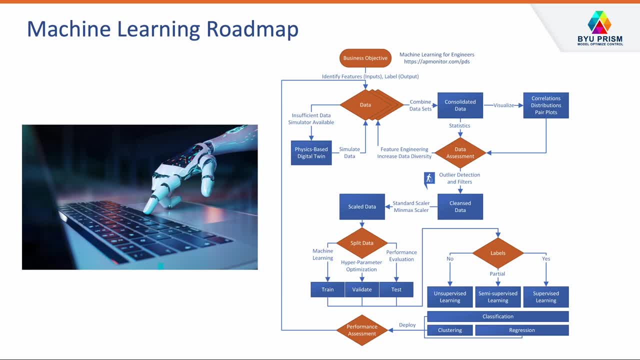 We get data, and if we don't have enough data, we might design and develop a physics-based digital twin to simulate more data. And then we combine these data sets, consolidate the data, visualize with correlations, distributions and pair plots, Also perform studies. 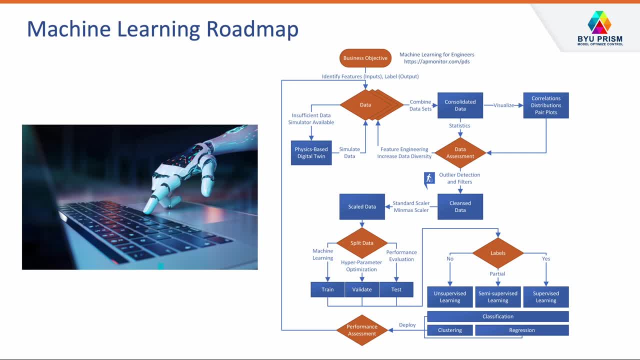 We do statistics on the data and then perform a data assessment. Do we have the right data to be able to solve this problem? If not, we do more feature engineering to increase the data diversity and maybe even combinations of the data sets to get new features and be able to meet this business objective. 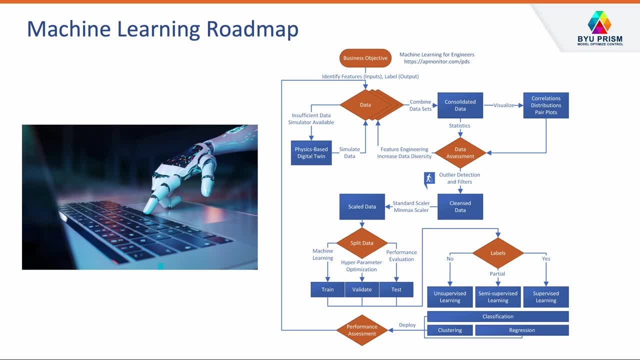 Then we go on to data cleansing, outlier detection and filtering and then scale the data with either a standard scale, Then we split the data into three sets for train validation and testing, And this is for the parameter updates, the hyperparameter optimization and then performance evaluation. 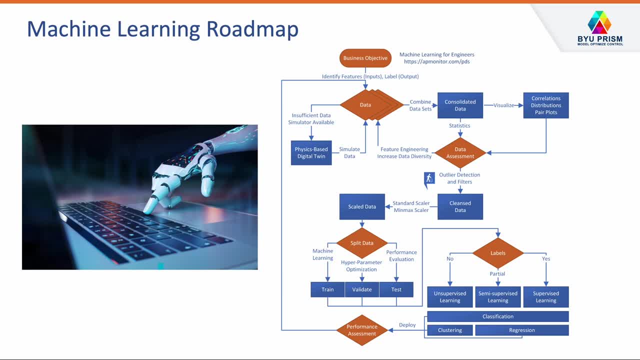 If there are labels, then we can do supervised learning. If there are no labels, then unsupervised learning, like clustering. If there's partial labeling, then we can do semi-supervised learning for classification or regression. So there are many data-driven modeling models. 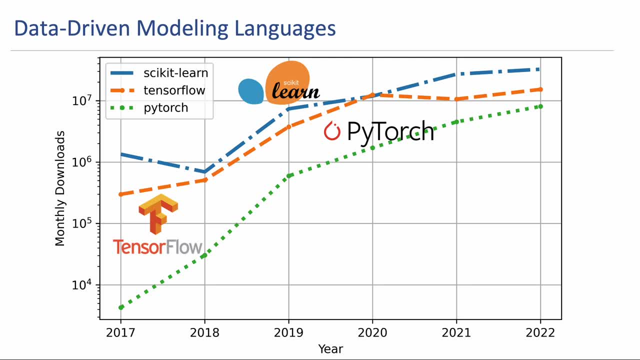 There are many languages like Scikit-learn, TensorFlow and PyTorch and others- Keras, that's a wrapper for TensorFlow. So you have these tools that have been increasing in popularity as data-driven methods have really been adopted more broadly. 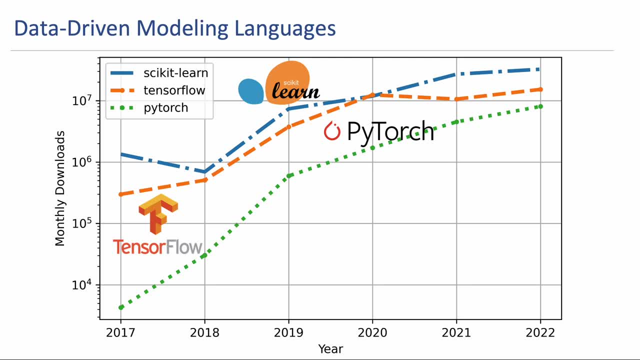 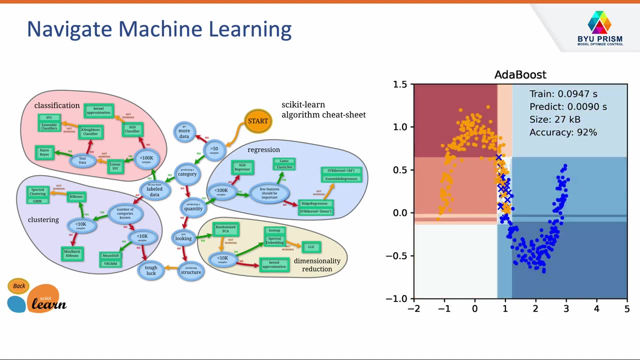 More people are using these. They're easier to use. They are creating interfaces even for auto machine learning or auto ML, to enable and facilitate machine learning, So you can use these tools to do all of these different applications. Really, what we need to be doing is architecting these solutions. 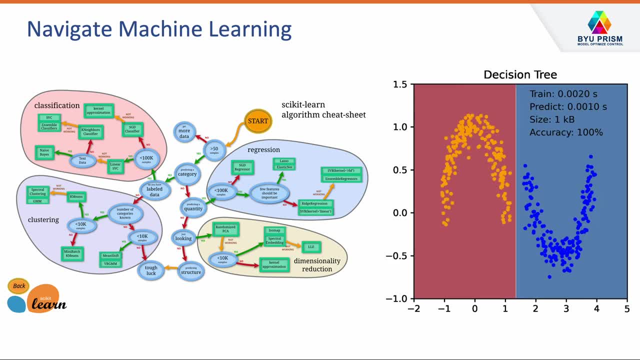 So, being aware of the methods, all of the classification and regression methods, so that when we're given a problem, we know: okay, these techniques are going to work well and these techniques won't. I need to be able to adjust the hyperparameters of this one so that it's going to work well. 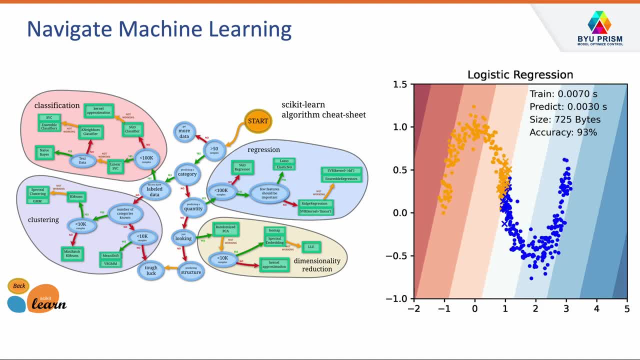 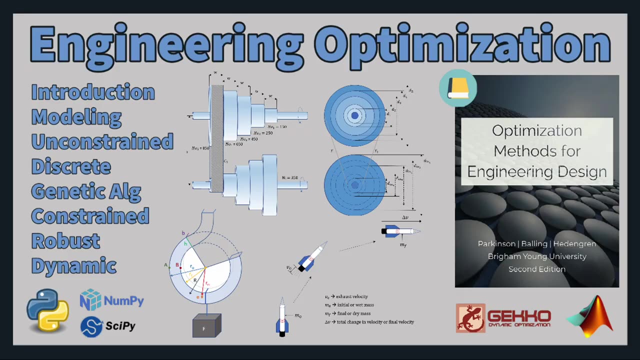 Alright. so there are different flow charts that we're going to go through To be able to decide what's appropriate: Regression, classification, clustering, dimensionality reduction- So many different things that we can look at with machine learning. Next, I want to talk a little bit about engineering optimization. 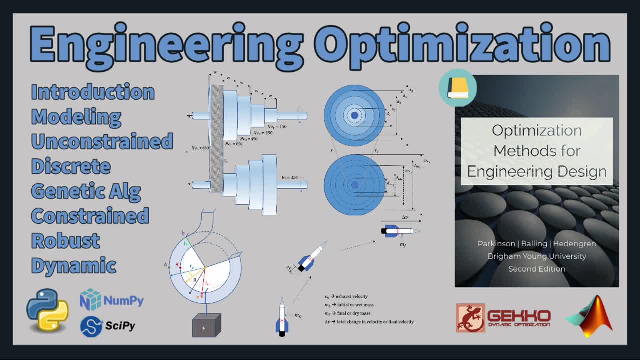 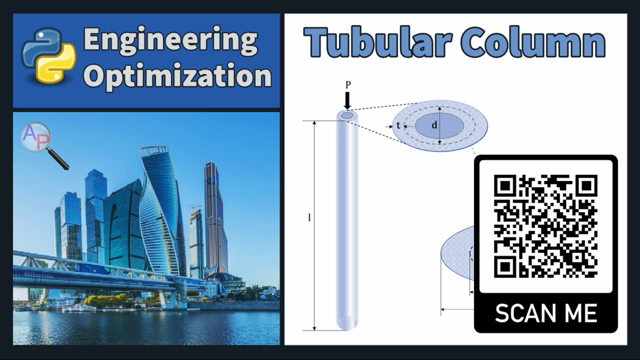 So this is a course where we really delve into the mathematics and of optimization, but also focus on solving optimization problems as engineers. So let's just take one example here, which is a tubular column, Designing the thickness and also the diameter of the tubular column to be able to meet a design specification. 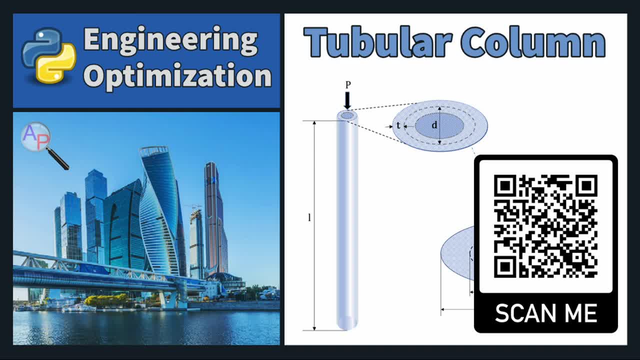 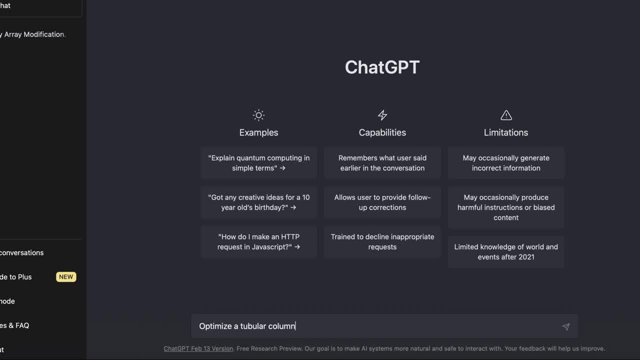 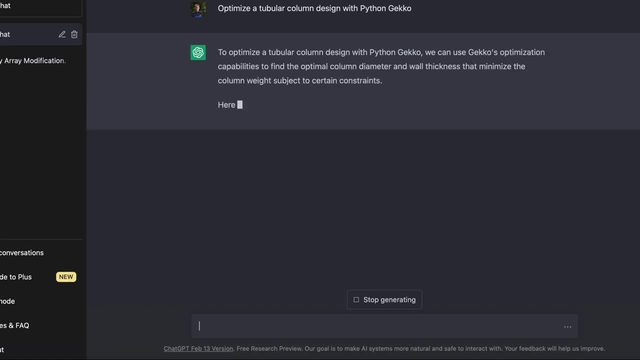 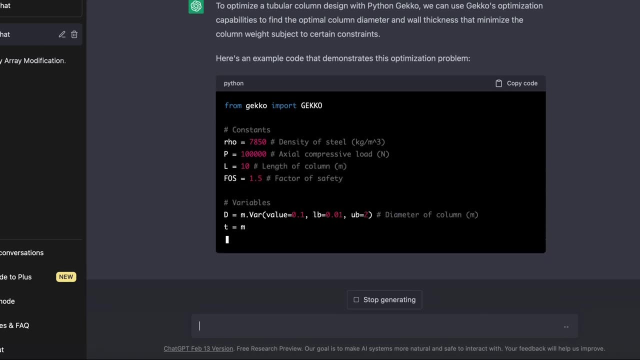 And I have a module prepared for this. but I also just wanted to see what chat GPT would do. Okay, if I wanted to optimize a tubular column design with Python Gecko, So to optimize we can use Gecko optimization capabilities. Here's example code that demonstrates this optimization problem. 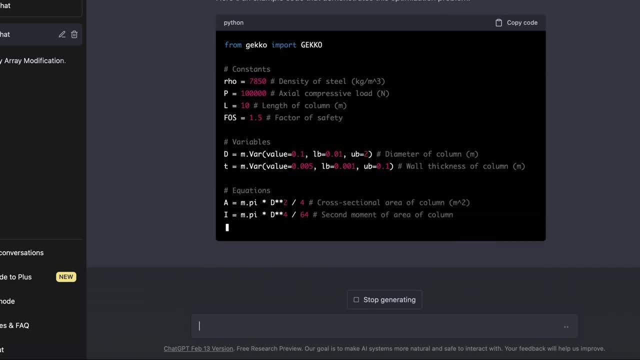 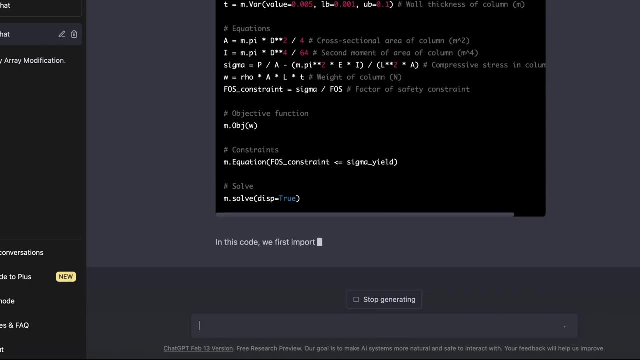 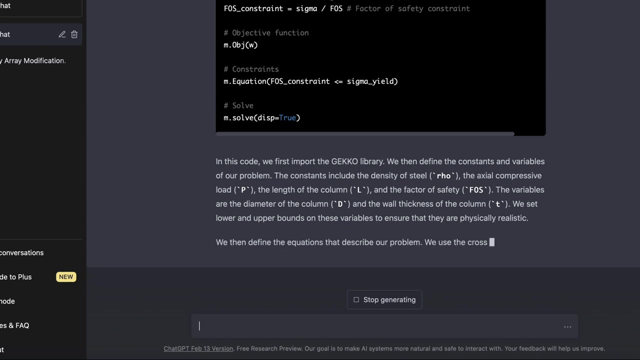 And I didn't tell it the diameter or the thickness, but it looks like it's learned from my course material or a similar problem to that: Set up and solve something similar, And I gave a description of the variables. Okay, So it did a fairly good job. 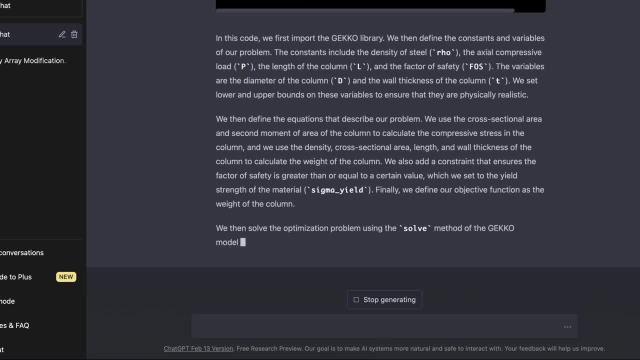 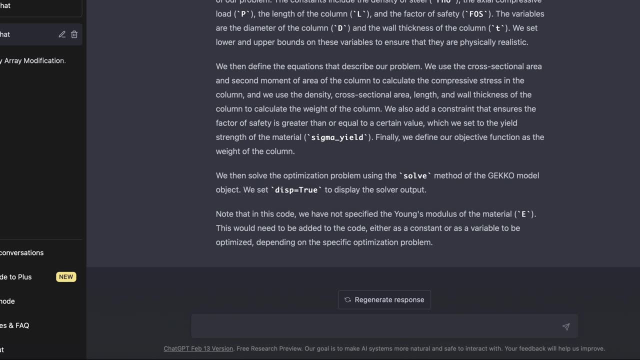 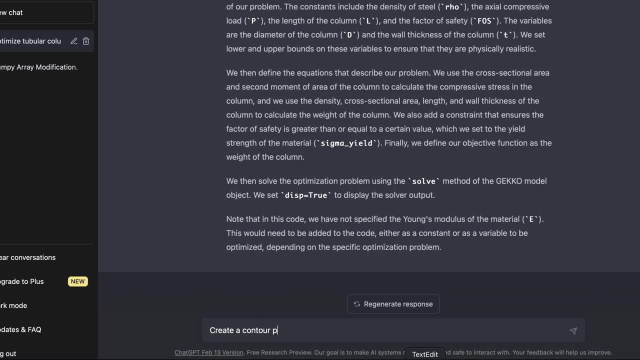 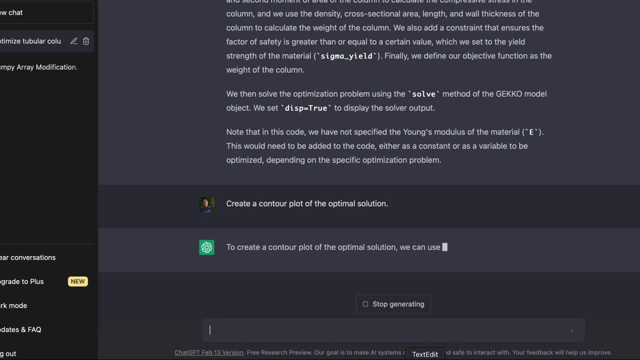 But other than that it looks correct, All right. but let's say I also want to create a contour plot of the optimal solution, So not just create the optimal solution but be able to visualize it. So this is going to give some suggestions on how to create the optimal solution. 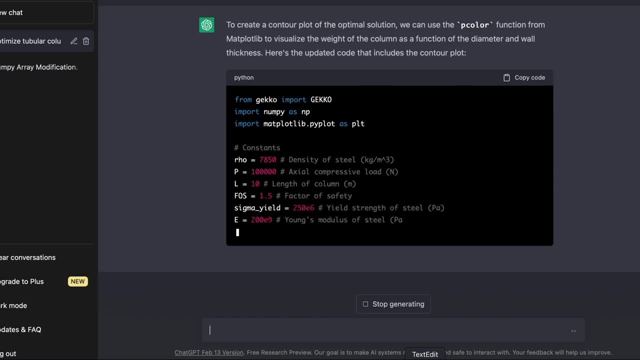 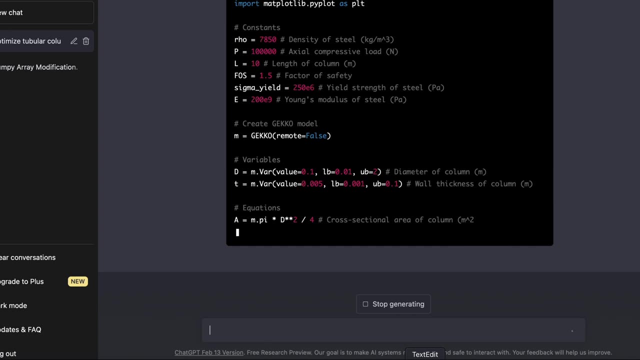 So this is going to give some suggestions on how to create the optimal solution. There's an option to create a contour plot as well. It's going to solve and set up and solve the optimization problem first, just like we did it before, But then it's going to now set up the contour plot as well, using a mesh grid to be able to evaluate it over all of these different scenarios. 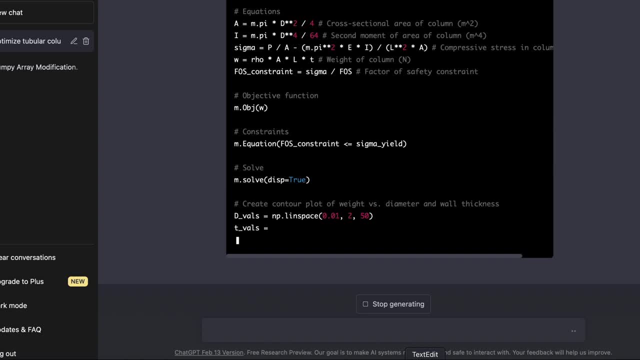 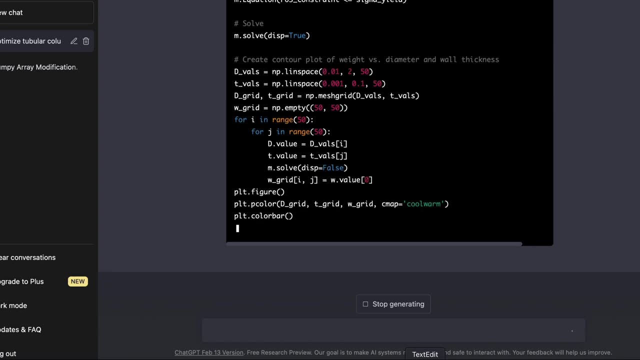 using a mesh grid to be able to evaluate it over all of these different scenarios and be able to create this contour plot. And again, it does an okay job with this. There's just a couple minor errors. There's just a couple minor errors and ID must be checked. 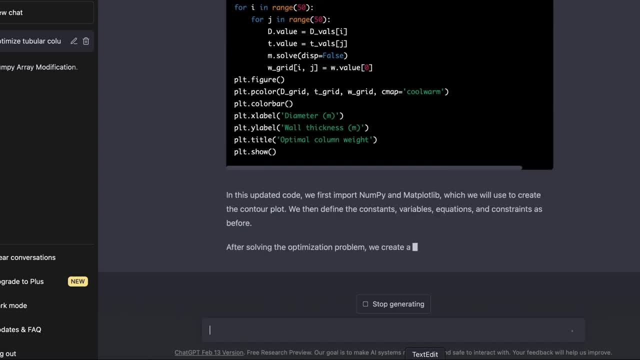 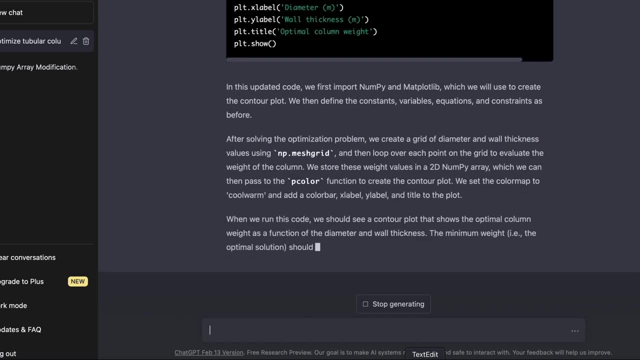 There's just a couple minor errors and ID must be checked. then I'll show the code that it comes up with, Okay. So, as I fixed a couple of these minor problems, okay, about four or five lines of code, it came up with this contour plot, right. 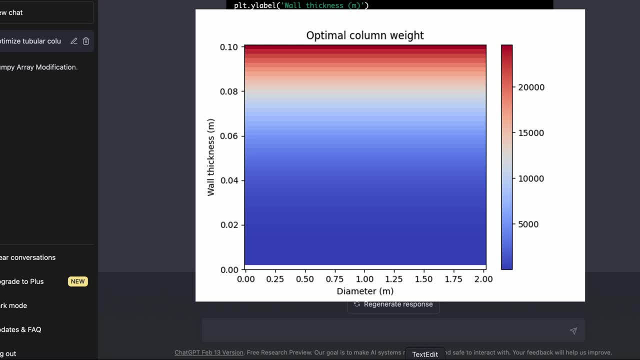 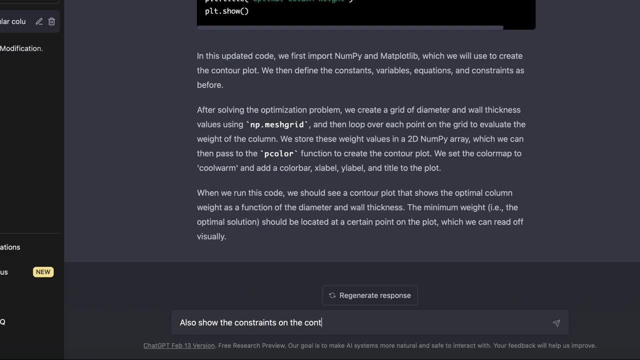 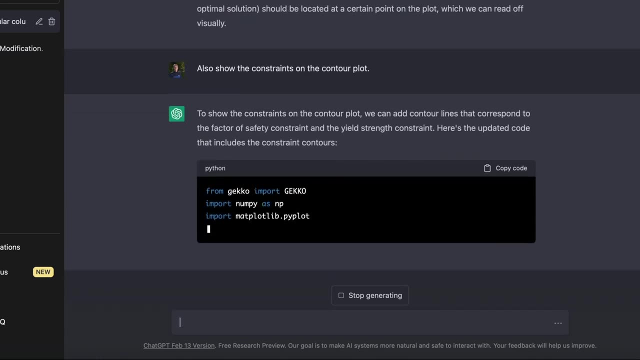 here with the optimal column weight versus diameter and wall thickness. But I also wanted it to include the constraints on that contour plot, to be able to show not just the objective function but also the constraints of the contour plot. Okay, So it's going to do it again. 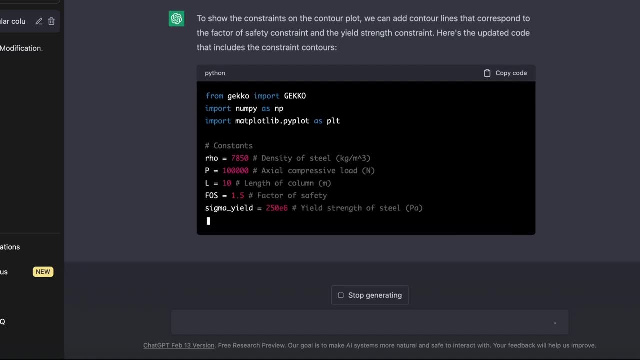 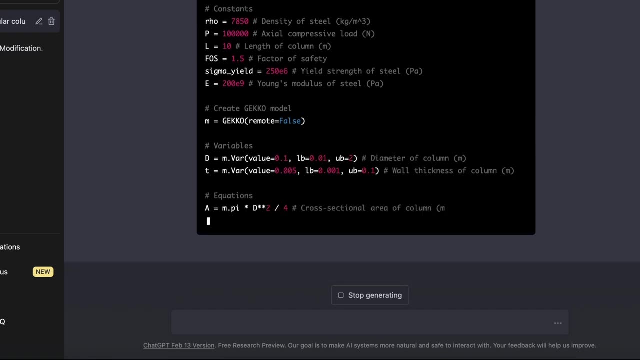 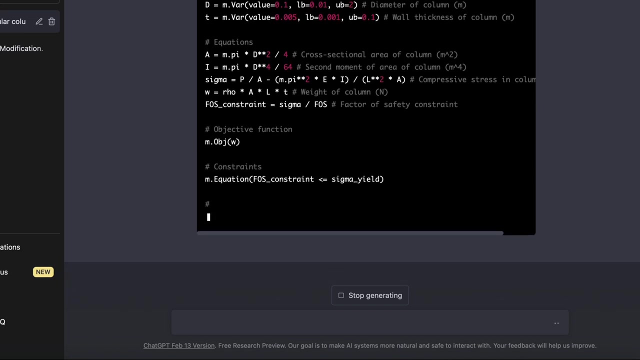 but add the constraints of the contour plot And I'll just show you know my solution for it. It didn't get it quite all the way correct. Plus, I wanted to add a couple other things on there as well, So I'll just show you my solution as well after this one finishes. But again, 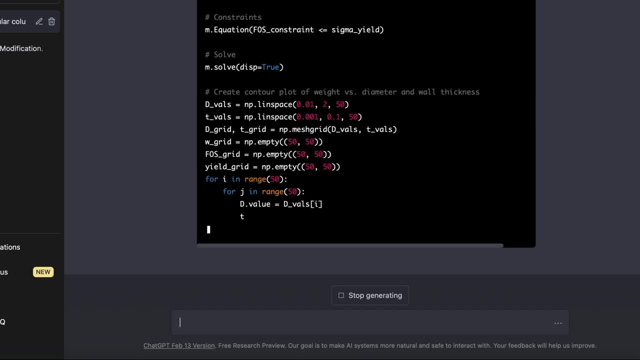 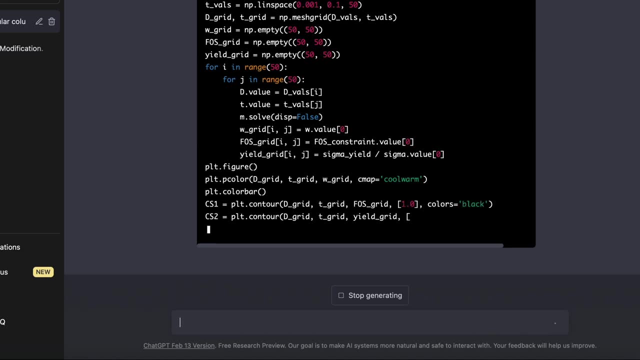 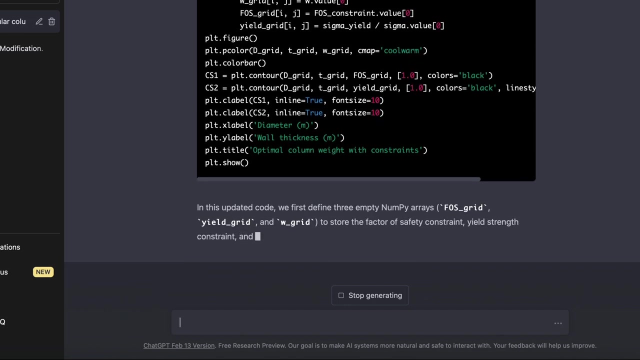 it gets fairly close, you know, in terms of solving an optimization problem, creating contour plots, be able to explain the solution. Okay, So there's its contour plot and explains a little bit about what it's doing in terms of creating it. All right, So here's the 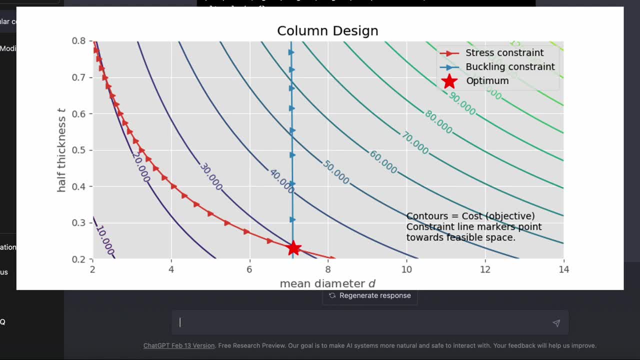 column design. There's the diameter and the thickness, And then this is my solution, not the one that it created. So I'll just show you my solution And then I'll just show you my solution that I created. but I want to show the optimum, So I could have continued to ask it for additional. 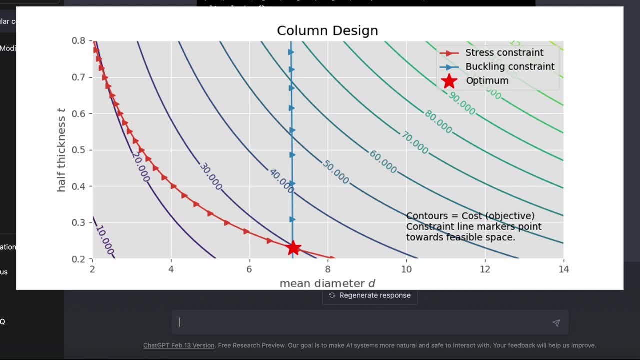 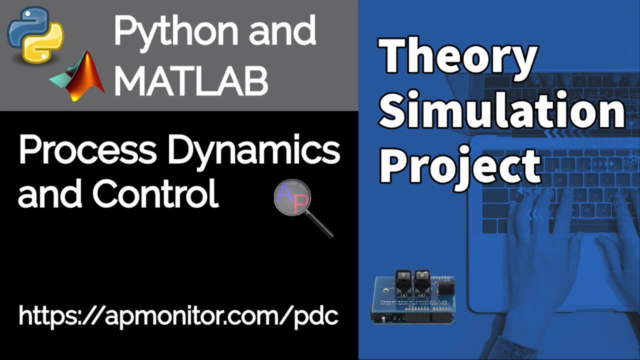 things. It would have been able to modify the code and then get it fairly close, But the star is where the optimum occurs, And then you have the buckling constraint and then the stress constraint there as well. All right, So let's go on to Python and MATLAB for process dynamics and 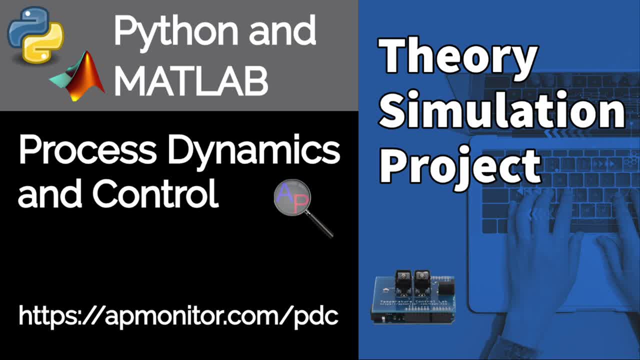 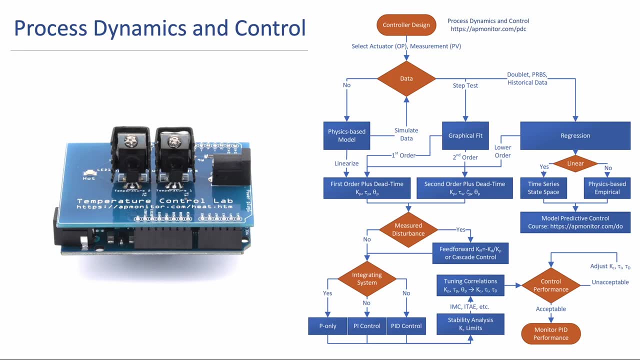 control. In this case there are live scripts, MATLAB live scripts, interactive, but also Jupyter notebooks and interactive modules in process dynamics and control and combining the theory simulation and the temperature control lab, And this one has a similar flow chart to the. 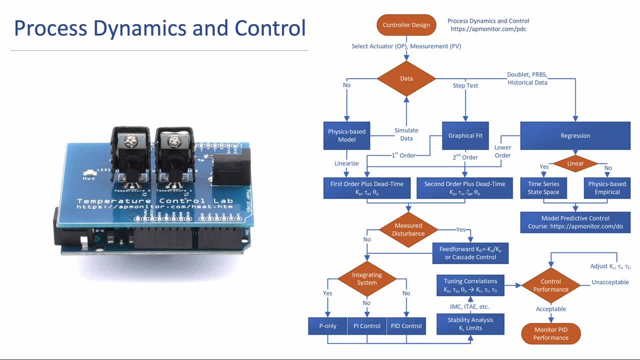 machine learning course, But in this case it shows some of the modeling up top, being able to create these empirical first-order plus dead time, time series, state, space or physics-based models and using graphical fit Regression or just the physics-based modeling to create these. Next, on the bottom part, if you have, 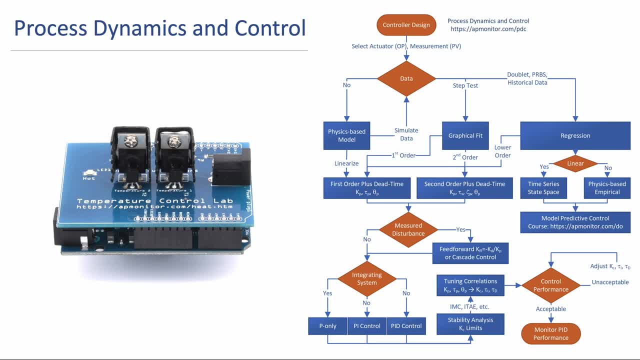 a measure disturbance, you might include a feed forward or cascade controller. If you have an integrating system, then you might choose a P only controller, but otherwise maybe a PI control or PID control. And even with an integrating system sometimes you do want a PI control anyway. 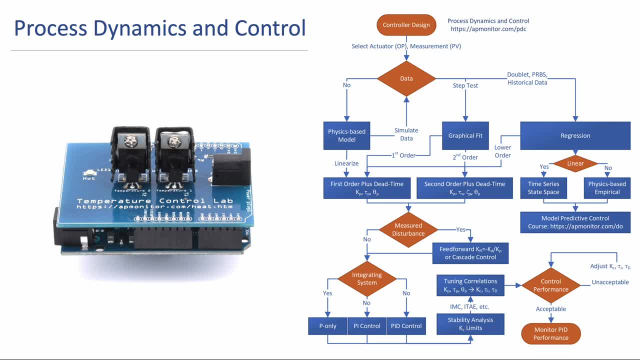 Stability limits and stability analysis, tuning correlations, control performance and then control performance And then you can continue to monitor PID performance. So really, this course is set up for introductory regulatory control. some of the theory and mathematics behind control: We use the temperature. 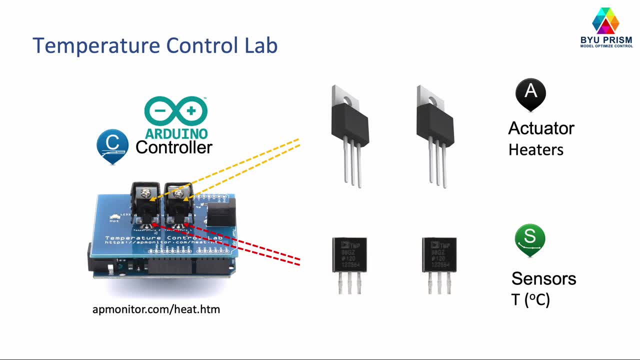 control lab as part of this. This little lab we've used at the university but also distributed it worldwide. There are 10,000 of these that have been produced. now about 70 universities that use this little lab to be able to reinforce concepts. 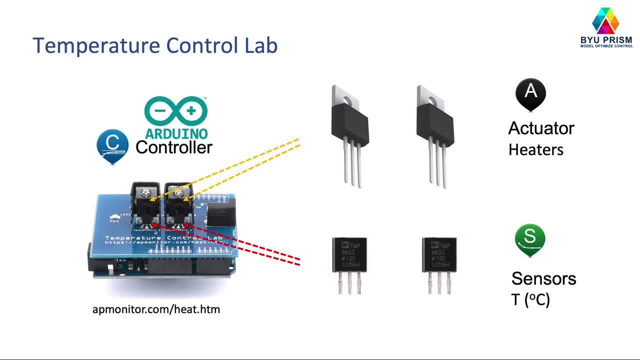 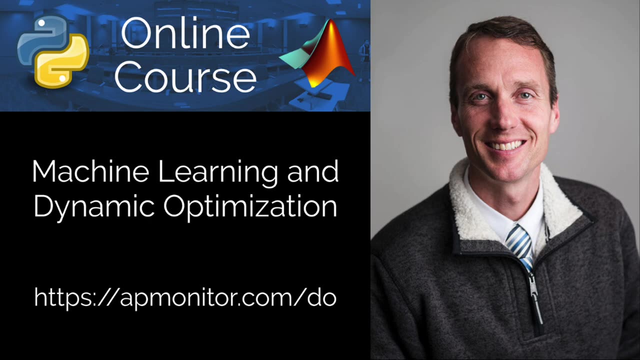 So we're going to talk about the data science, machine learning, control theory and others. It gives two actuators, two sensors and a simple multivariate control problem. So let me just talk a little bit about the machine learning and dynamic optimization course. This one's a. 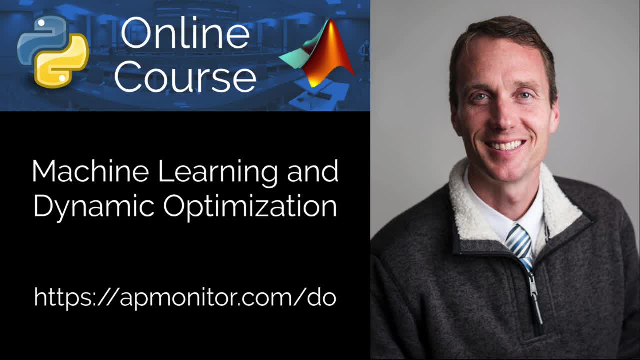 graduate level course that combines optimization with dynamics, to be able to design systems that have differential and algebraic equations, or machine-learned models that have some kind of a time-bearing component to them, like an LSTM or a transformer that you want to be able to use in a model predictive controller. 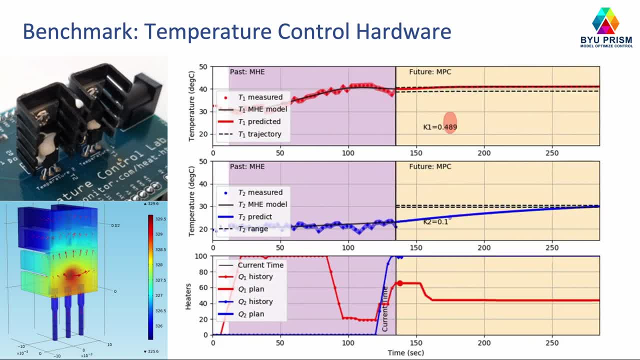 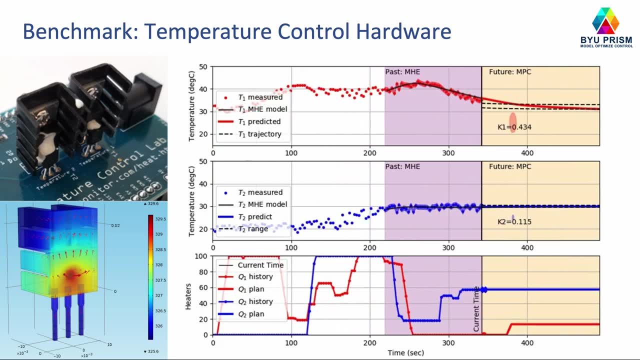 So in this course we discuss concepts like moving horizon estimation- that you can see in the purple- or model predictive control as well, And then again we also use the temperature control lab, in this case to not only have a theoretical treatment of these topics, but also to 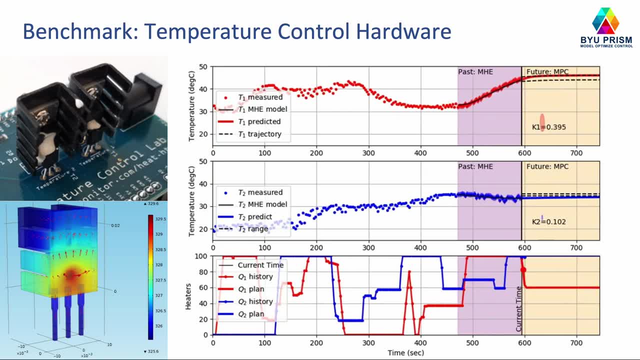 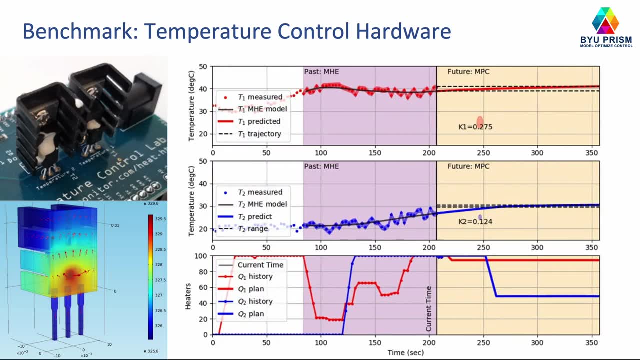 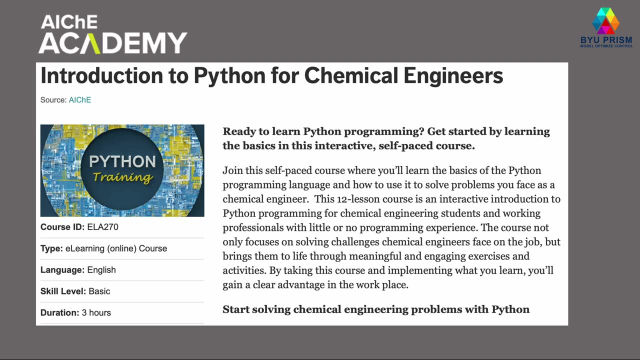 be able to apply it to a real physical system where every student has their own lab. that's slightly different and they get to work with it to do the modeling, estimation and control. I also want to mention- this is a common question that I get- is about getting credit for these courses. 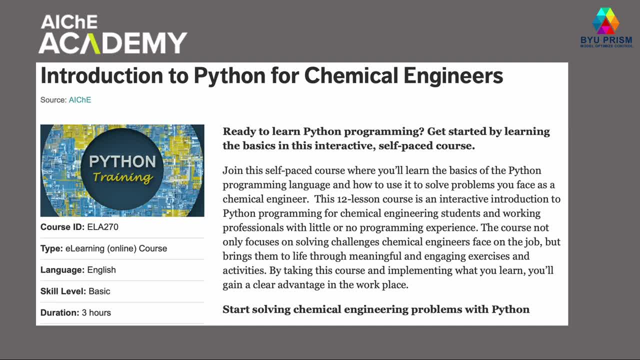 Now all of these courses are freely available on the website- the apmonitorcom website- but I also got many requests to be able to offer these for the professional development hours or continuing education units that many professionals need, And so we've partnered with AICHE, AICHE Academy, to make these courses available there as well. 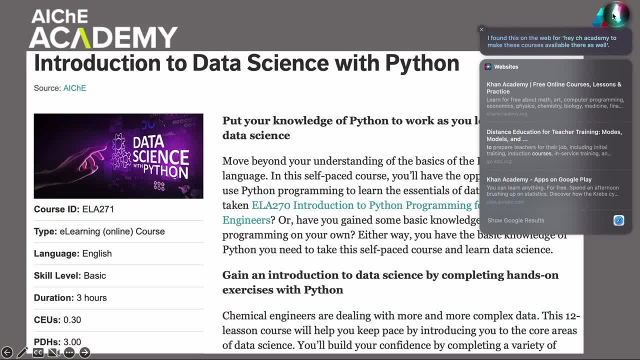 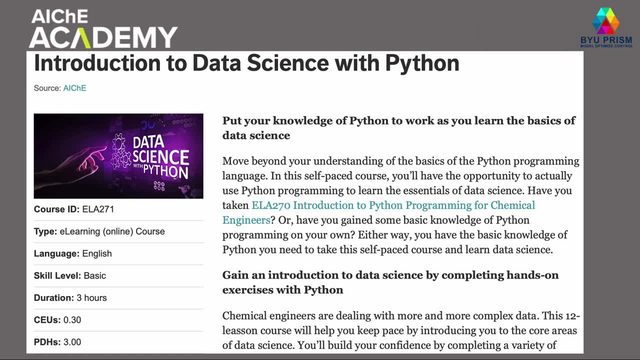 Okay, I found this on the web for AICHE Academy to make. I don't want that. Okay, let me close that out. Fine, I think it. It triggered my Siri. Okay, so this is another one: Data Science, with Python as well. 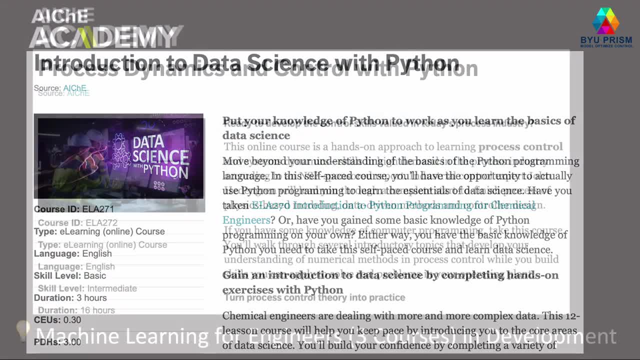 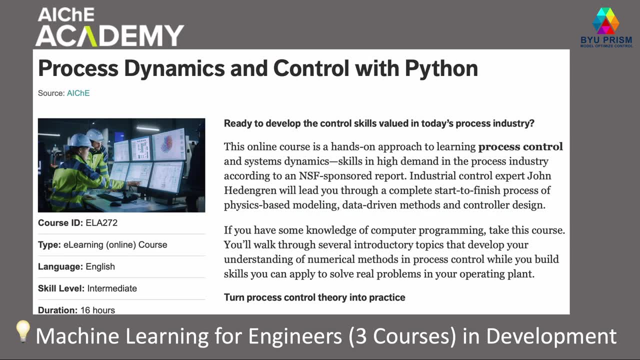 And I just want to share with you that these courses- we have these three available right now, but three additional ones are going to be made available on machine learning. So those are coming for machine learning for engineers. They've broken it into three modules. 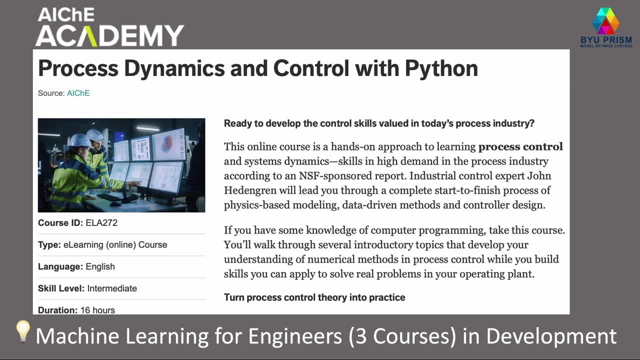 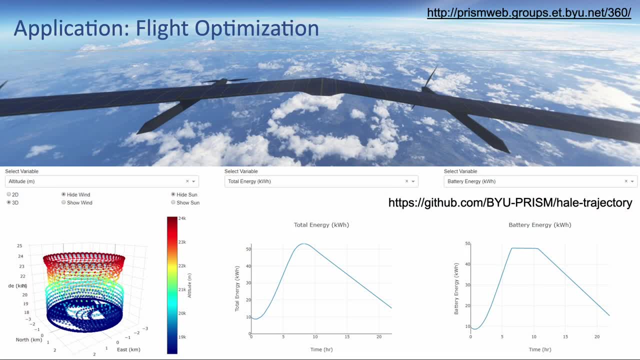 They've made it a little bit easier to make it through the course material. Okay, so now we have an application of. I'll talk a little bit about my research. So this is. These are some of the projects that we've worked on and it relates to how we do this. you know: data science, machine learning, dynamics, optimization model, predictive control. 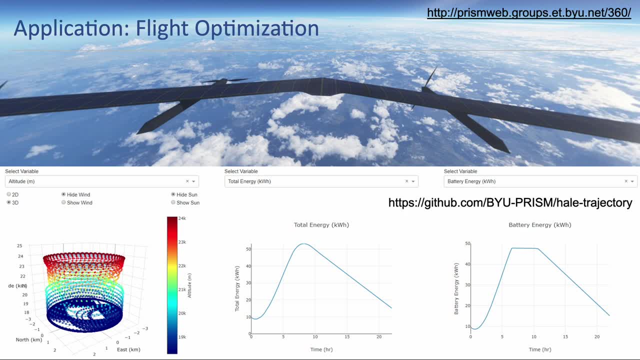 So each of these projects use Okay, data science, machine learning, dynamics, optimization, model, predictive control. So each of these projects use some of those, and one of the hallmarks of working with students is especially at Brigham. Union University is that we have about 90 percent of students who are undergraduates, who are involved in research, and about 45 percent of them are co-authors on publications, and BYU is. it depends on the year, but we're often in the top 10 for number of students that continue on to graduate. 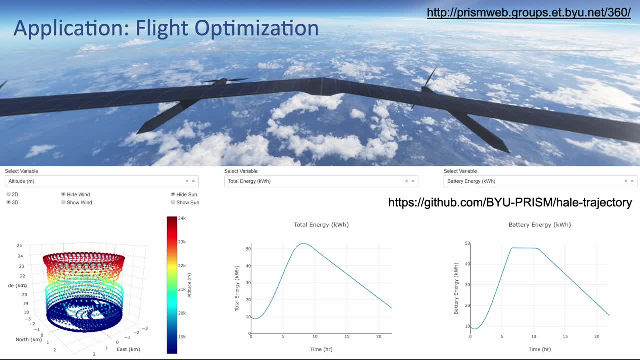 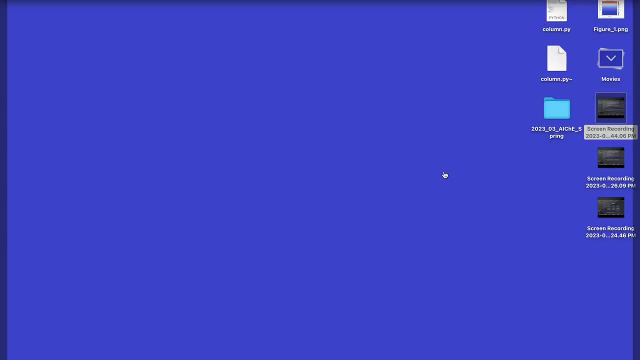 school and one year we're fifth, so we're one of the top universities that send undergraduates out to get a graduate education. part of that reason is that so many of them are involved in this experiential learning. this is just one example of a project. I'll go ahead and just open this up. 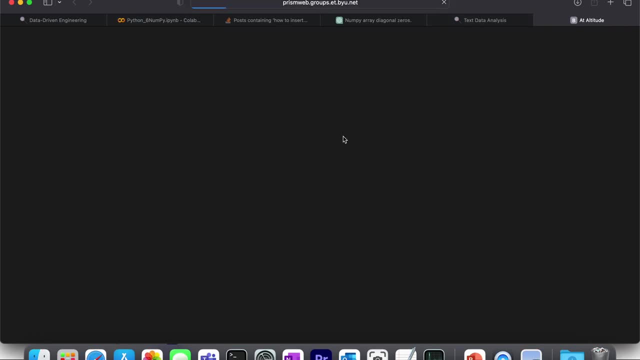 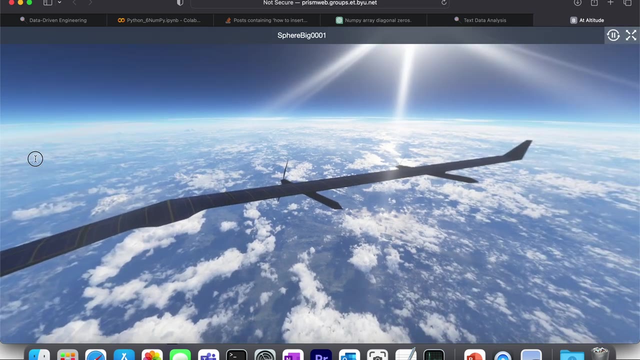 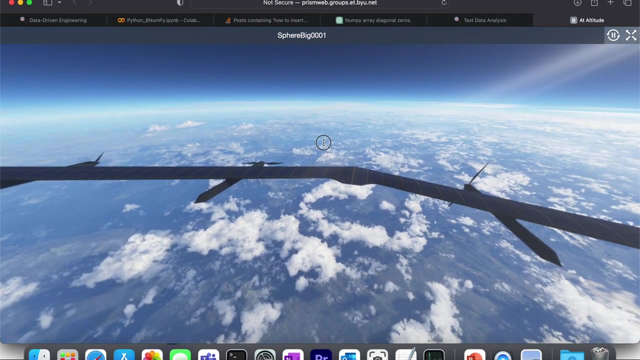 okay, this is the the flying wing. okay, a UAV that's meant to of the flying wing. okay, a UAV that's meant to deliver internet to remote parts of the world about as wide as a 737 aircraft, colored in covered in solar panels. the objective is to try to stay aloft- 60,000 feet elevation- even during winter. 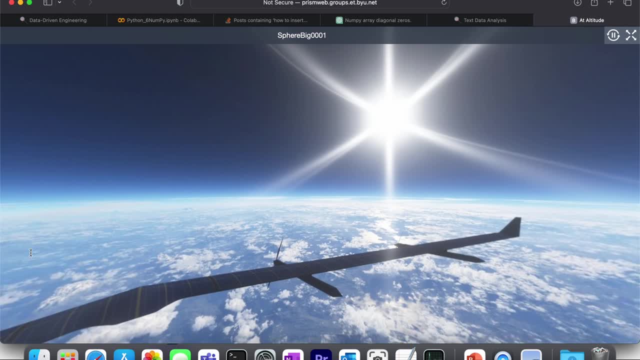 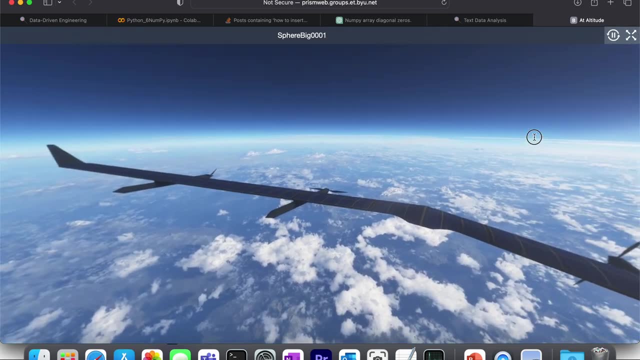 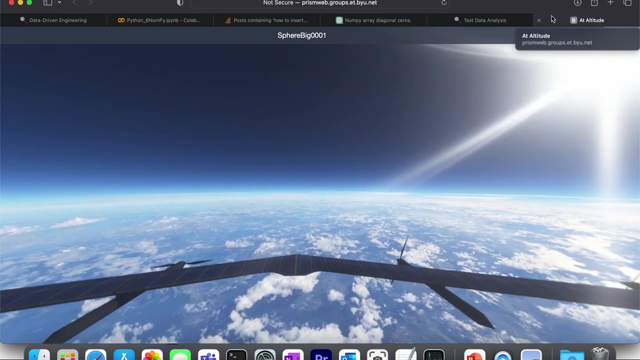 solstice- okay, so the most challenging time of the year, at 42 degrees north latitude, and when we were first given this problem, we could go about 17 hours and it you know we we didn't have enough energy to be able to stay aloft during the night time, and so we gave this to an optimizer to be. 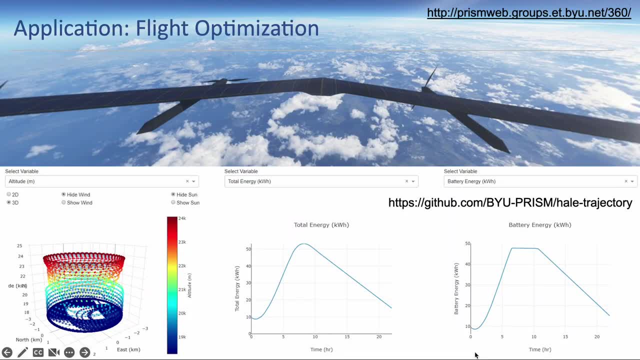 able to determine how to fly more optimally, and it did something you could see here in the left: it started flying not just in a circular orbit, but it flew in a way that was banked toward the sun and somewhat of a a modified oval shape, and it was able to collect more solar energy. and when his battery was full, 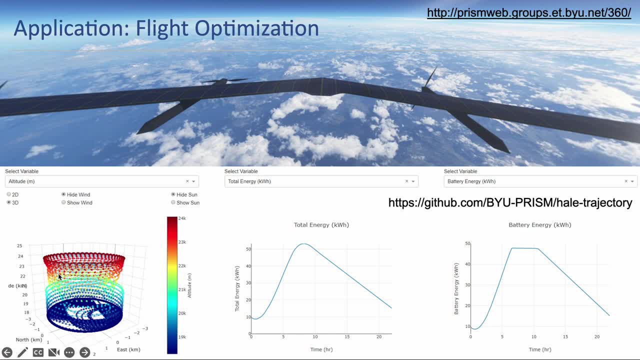 then it climbed in elevation, so it climbed to be able to store the potential energy when its battery was full, and it was able to figure all of this out by using these optimization algorithms combined with these physics-based digital twin of the aircraft to be able to navigate it and perform these scenarios. for it to be able to fly, it was able to be able to get up to 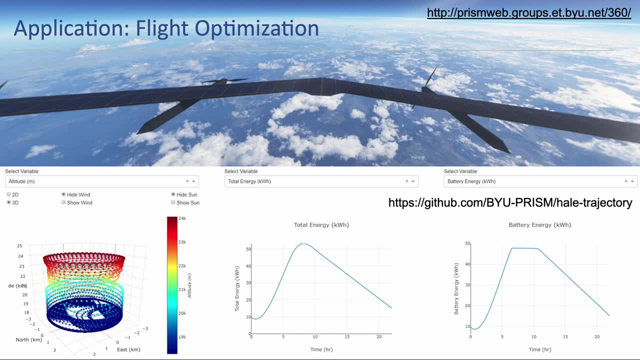 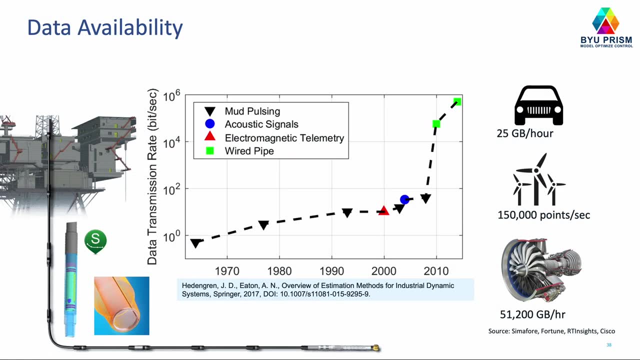 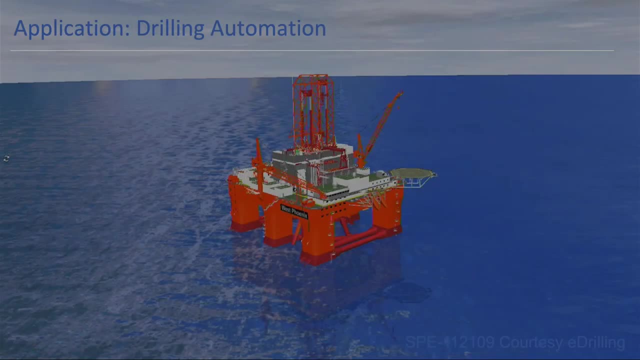 this 24-hour target, to be able to stay up even during winter solstice at that challenging latitude. also, we've worked on data drilling and how to use technologies like wire drill pipe okay- that have increased the amount of data that is available downhole, and this is a çu走. 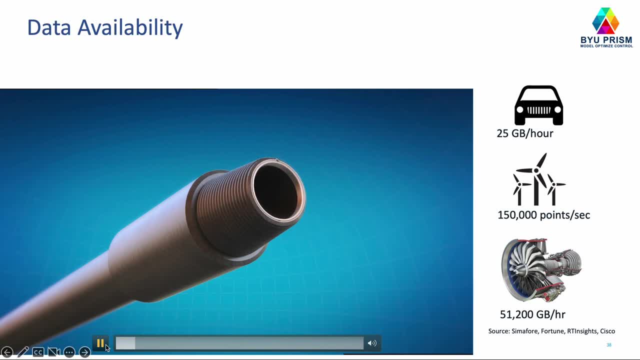 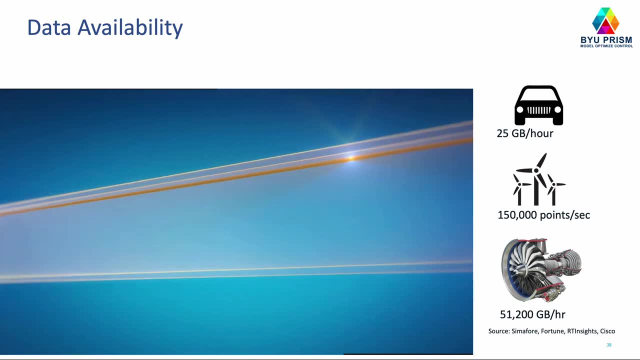 vor a outflow somewhere in here. wу is analogous to what's happening in many other industries And you can see some examples there on the right, with self-driving cars, maybe 25 gigabytes an hour, a wind farm, 150,000 data. 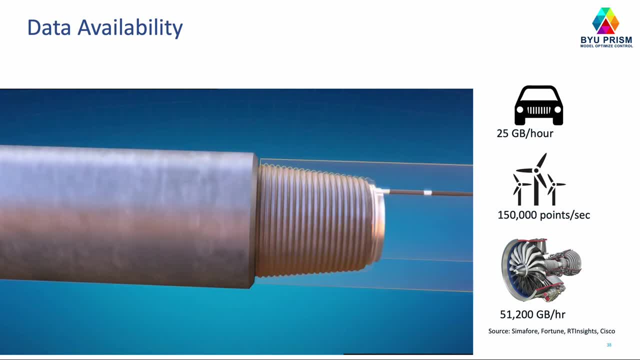 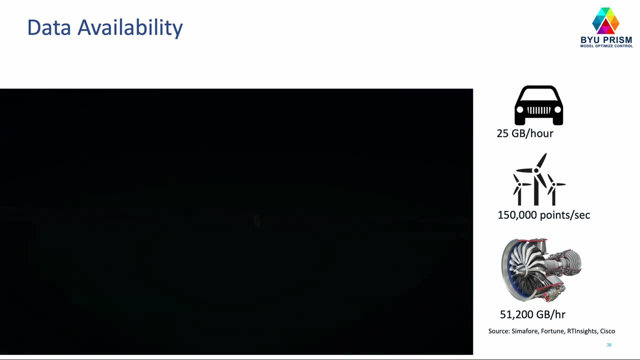 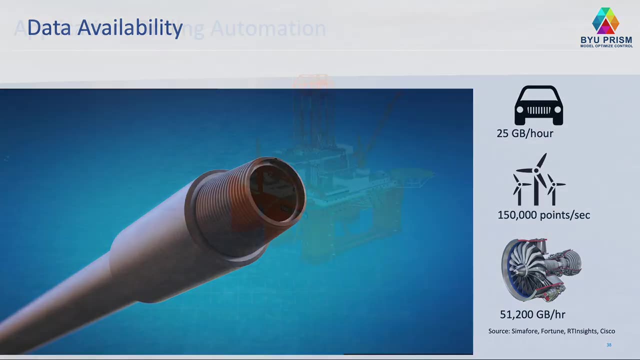 points. a second, you know: turbine on a jet engine about 51,000 gigabytes per hour. So in each of these cases there's a lot of data availability And what the challenge is is how do we take that data and turn it into actionable information. So we've also worked on drilling automation using 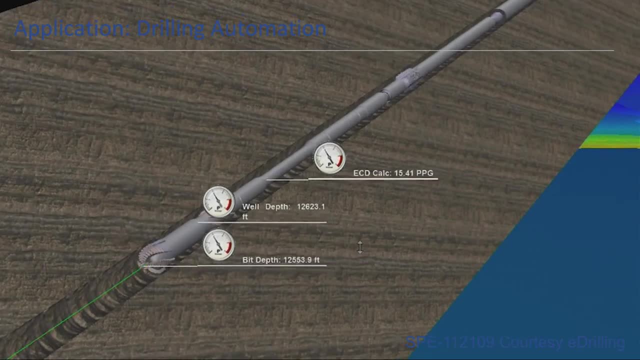 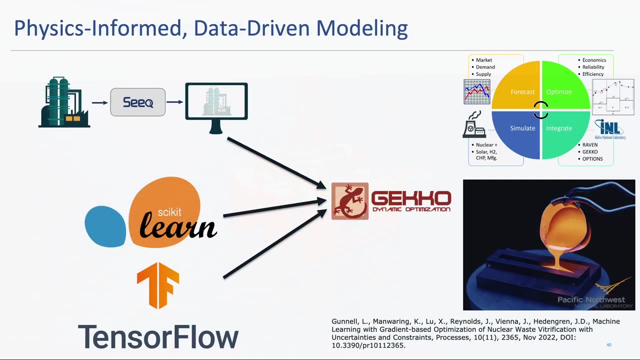 these very complicated physics-based models, And how do you create simplified models that can be used in control and automation? Another thing that we've been working on recently is being able to combine the power of optimization and control with some of these other packages for machine learning. 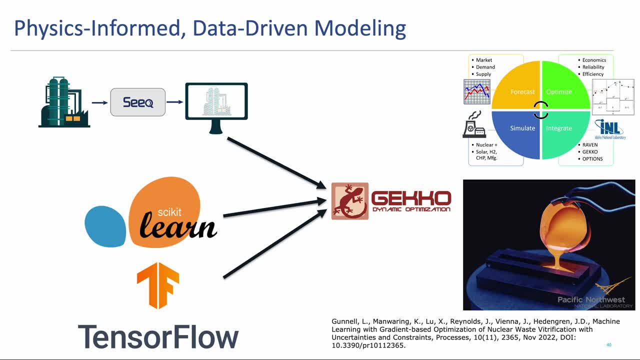 and data science, Like Scikit-learn with TensorFlow as well. So a support vector regressor can use that directly in an optimization problem, much like that tubular column where you might have part of the design that is determined from a regression, for example. Also, we've been partnering with Seek to be able to make 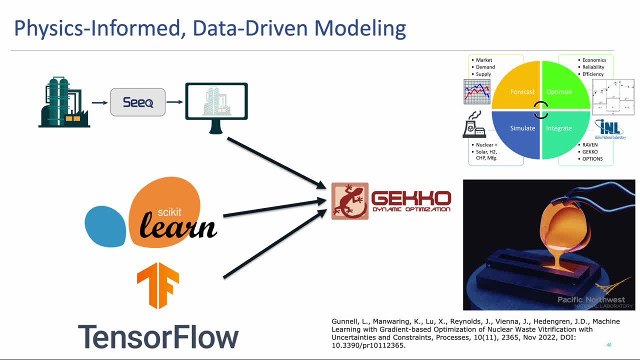 some of these developments easier to use through a graphical user interface, through Jupyter notebooks that are open source, And applications As well in vitrification of nuclear waste, with Pacific Northwest National Labs, Department of Energy, on some forecast, optimization, simulation, integration and the smart grid systems with small modular reactors. 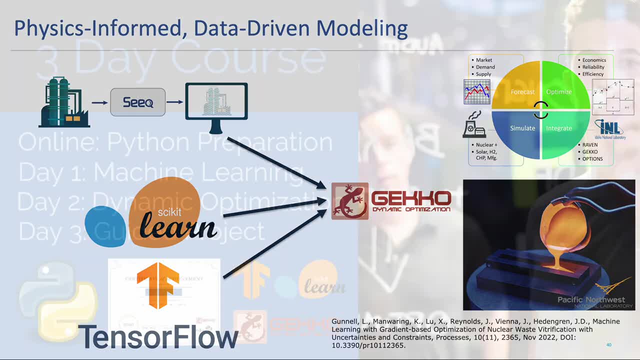 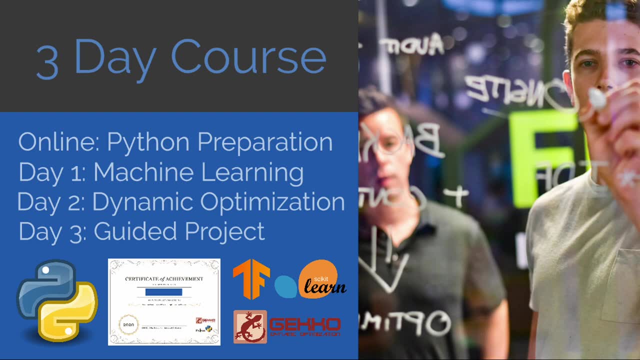 and other applications revolving around energy. I'll just mention we've gone through some of this course material. There's AICHE Academy- all of the course materials online- But sometimes an organization needs something just a little bit more And we found that going to the company and working with them directly over an extended period of time. 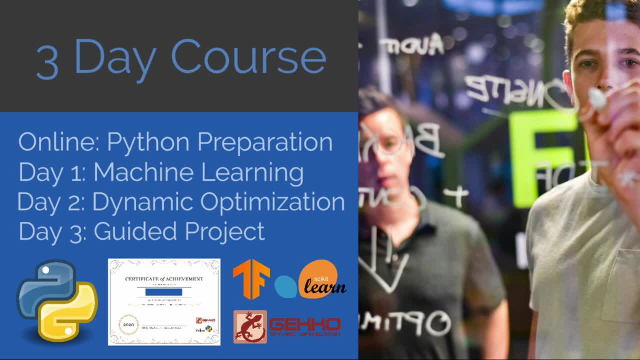 maybe three days with a short course or maybe regular update meetings, has really helped to upgrade a whole organization to use some of these new tools and be able to start exploring, Because really you want to be able to give these tools to those who are most familiar with their. 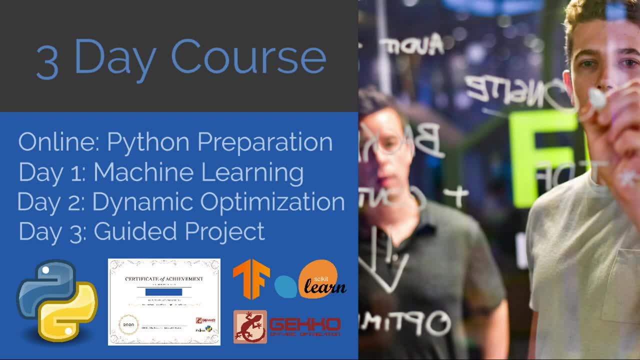 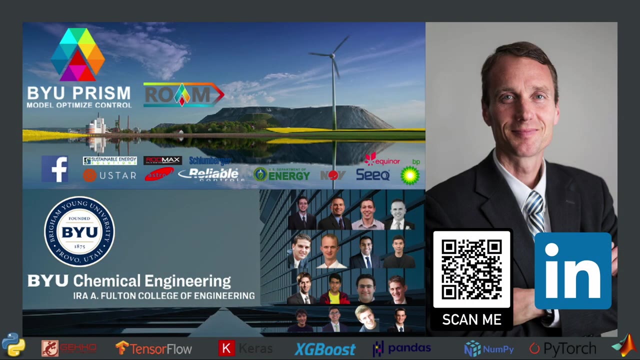 process. that's where the impact happens, is where they have new ways of analyzing data, be able to create new applications and get those applications online, so they start making automated decisions. I'll mention just a little bit about my research group as well. I really appreciate all of the 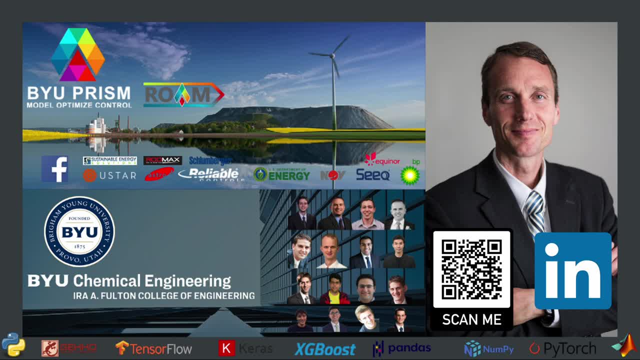 graduate students who have contributed so much to this research. as a professor, a lot of times on the face of the group, gets to promote their work and the excellent job that they're doing to be able to create these innovations, new software packages, new capabilities. so I really 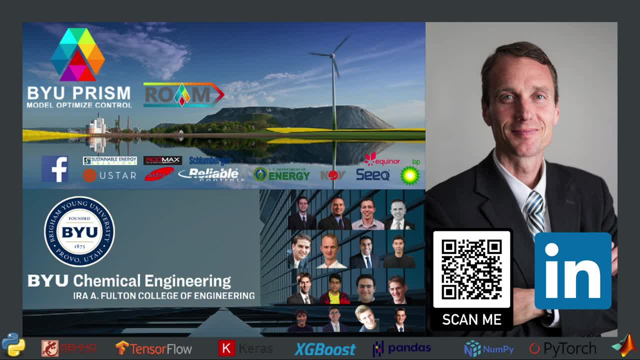 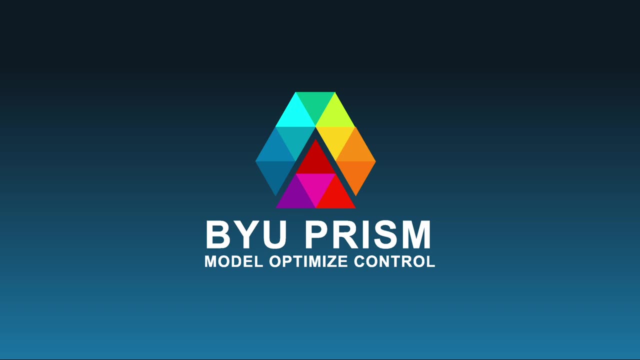 appreciate their work as well. I also like to be able to connect with you on LinkedIn, so there's a QR code to be able to connect with me on LinkedIn as well. so thank you for your attention and I appreciate this opportunity to share some material about the courses, my research and also a